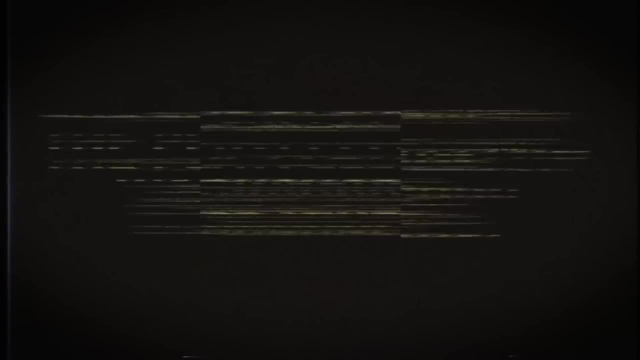 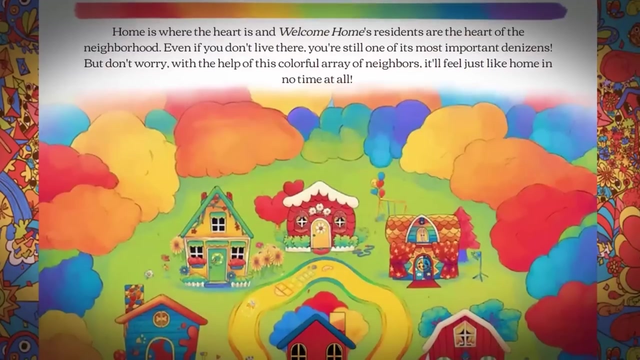 A kids' educational series that suddenly went off the air and disappeared. Even its production company went completely silent. In that way, it's very reminiscent of Hello Puppet, If you happen to remember that one. As we explore the website, we can learn more about the residents of the neighborhood called Home. 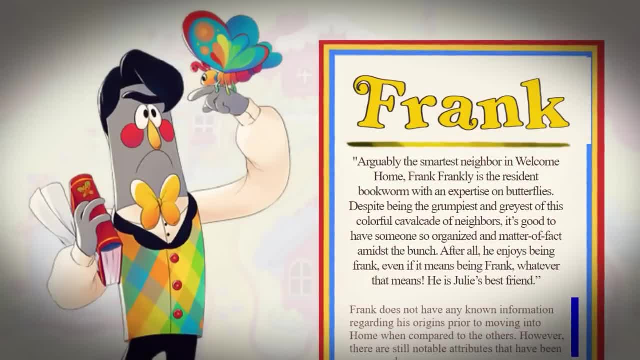 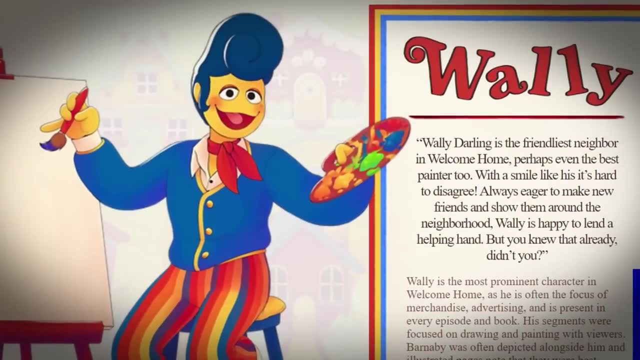 And it's your typical Children's Edutainment roster: People like Grumpy Frank, Joyful, Julie Goofy, but Streetwise Barnaby. but the most important character is the lead, Wally darling, A character who's one part Mr Rogers, one part Sesame Street, with just a dash of Bob Ross thrown in. 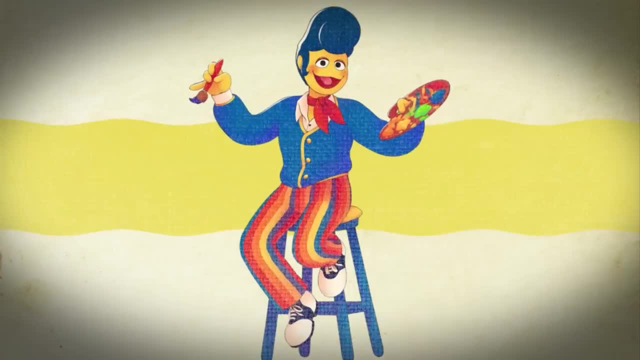 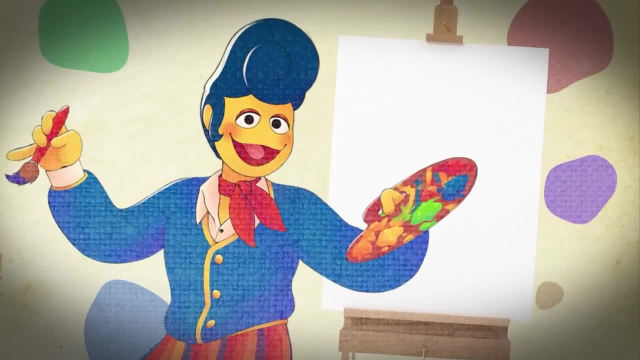 because the Internet do what the Internet gonna do. Exploring the website, we learned that episodes of the show would revolve around Wally learning a lesson, going on adventures and drawing and painting with viewers. It all sounds quite idyllic, really. 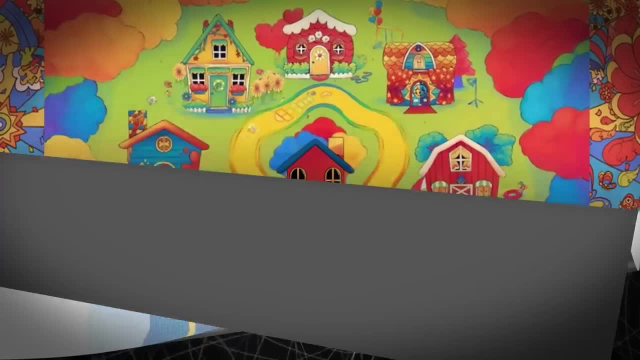 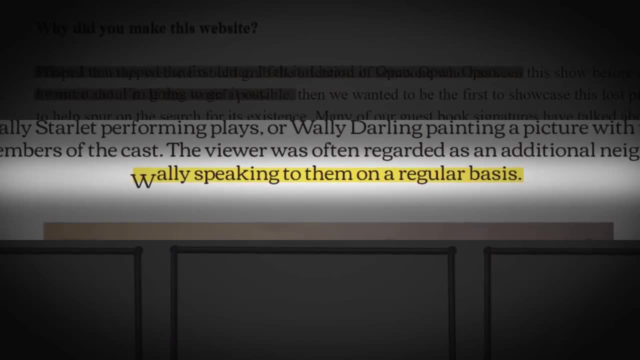 And it is at least until you look beneath the surface. As you explore the website, you get a sense that not everything is right in this neighborhood. Links don't seem to work as they should. text appears to be overlapping out of alignment or hidden entirely. 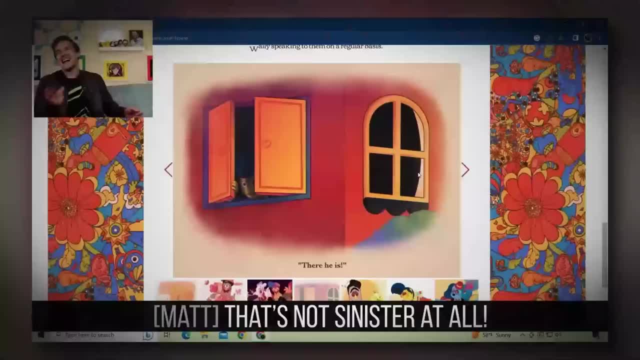 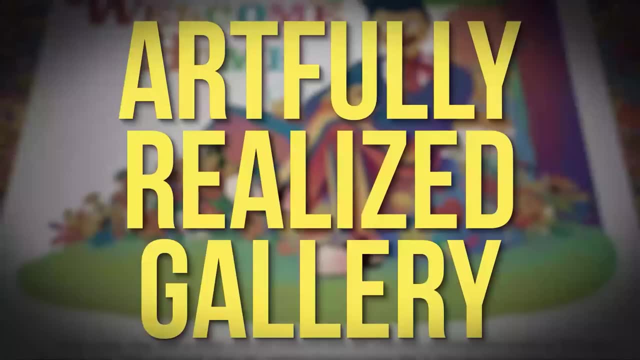 and there's this weird image of WALL-E just looking mighty sus. That's not sinister at all. There he is. Ladies and gentlemen, this isn't just a website. it's an ARG, An artfully realized gallery full of drawings, cardboard models, vinyl records, a physical puppet. 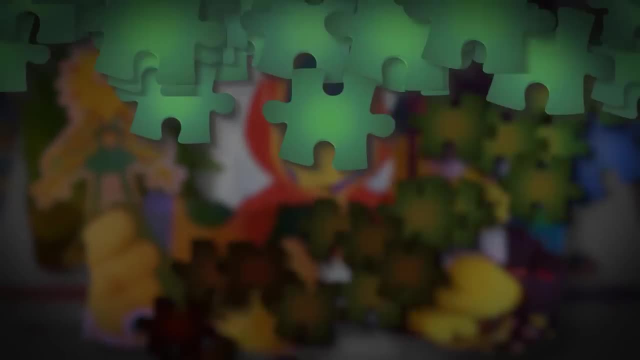 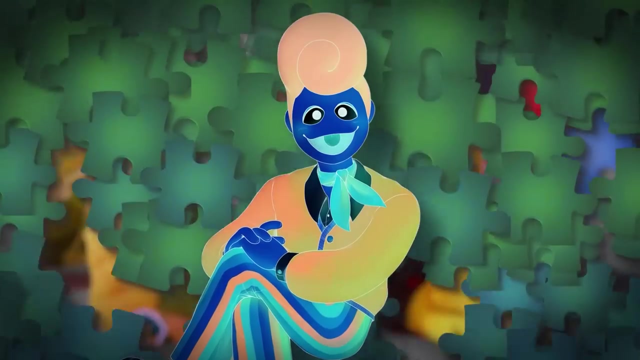 and, of course, puzzles, Lots of puzzles, And they're all hiding a suspicious amount of LORE. Something sinister is going on in this neighborhood and we're about to figure out what it is. But before we dive in, I do want to take a minute to remind everyone that 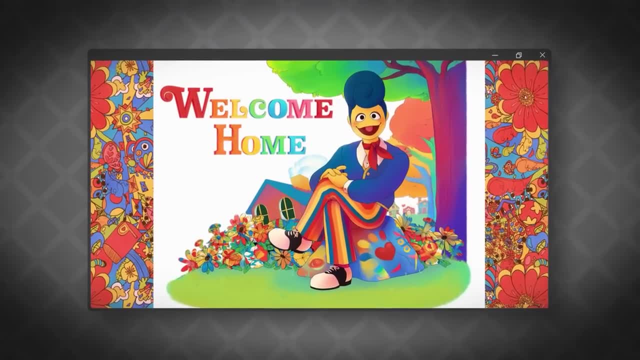 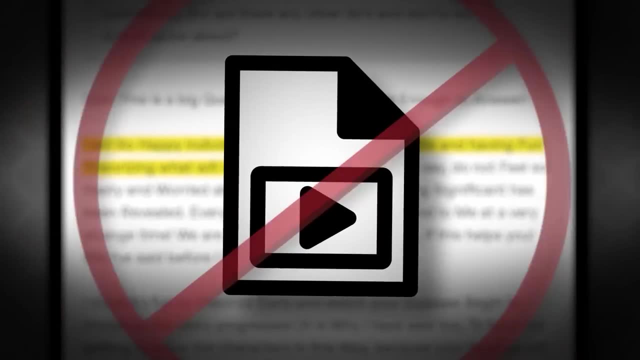 while, yes, websites with secrets like this are exciting, we have to be kind and respectful while we explore. Welcome Home's creator, Clown, has been very explicit in saying that they welcome theorizing, but they also ask that you don't share them on any theory videos, for fear of the video influencing their intended narrative. 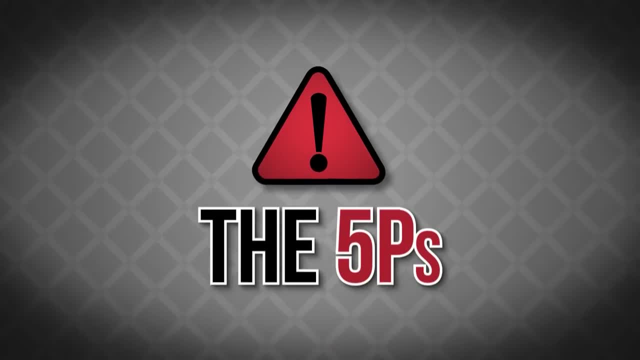 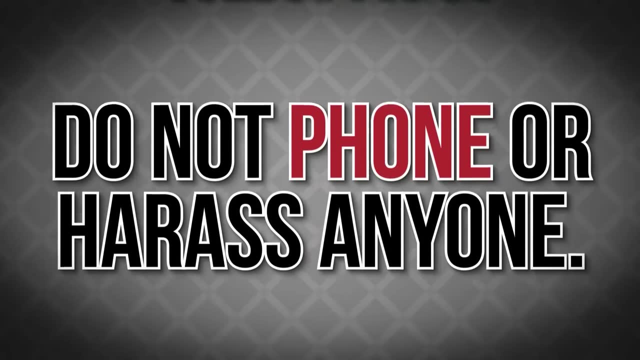 Additionally, as always with any website-based mystery, remember our five rules that we've covered in past episodes: Never publish private information, stick to publicly available information, do not trespass, do not contact or harass individuals and keep the discussion centralized. 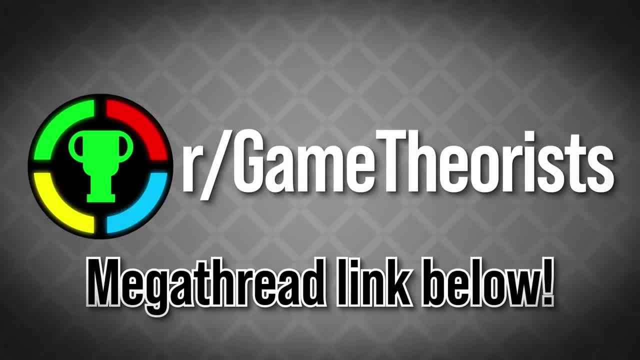 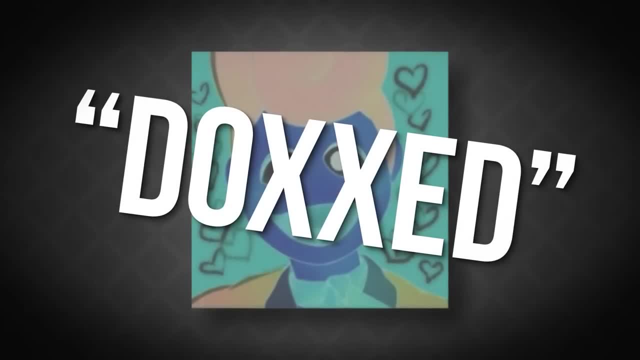 To help with that, there's gonna be a link in the description for the mega-thread on the Game Theorist subreddit. But these rules are especially true for this particular series. Rumors have been circulating in the community that Clown has actually been doxxed. 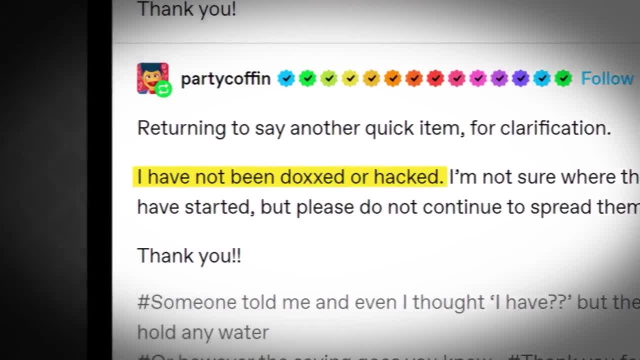 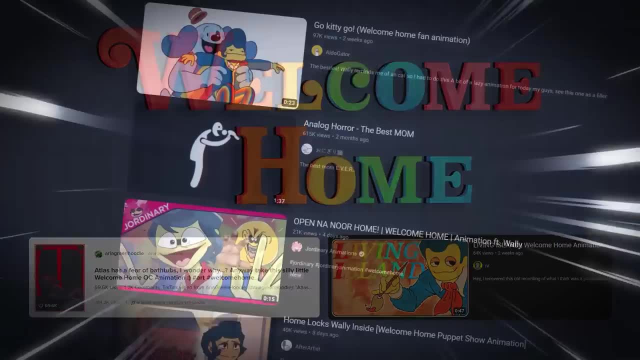 Fortunately, they put out a post confirming that that isn't true. that said, let's just keep it that way. Secondly, as I mentioned before, online discussion about this world and its characters has blown up across TikTok and YouTube, And because of how quickly and aggressively this has gained in popularity, 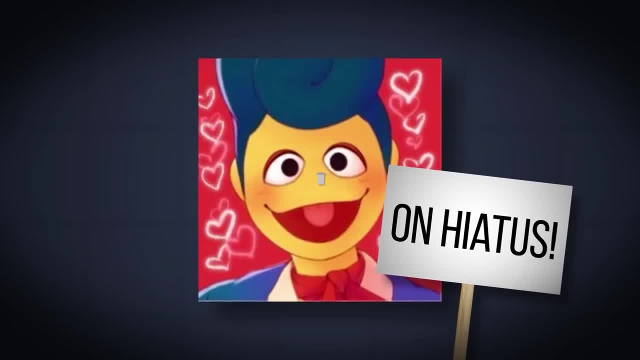 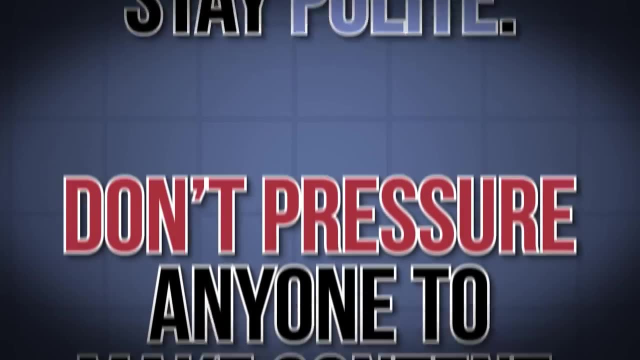 Clown's currently taking a step back from posting and creating. right now There's even a deleted post saying how overwhelmed they feel by the amount of attention the project's received. So, just as a reminder, stay patient, stay polite and do not pressure anyone into making more content. 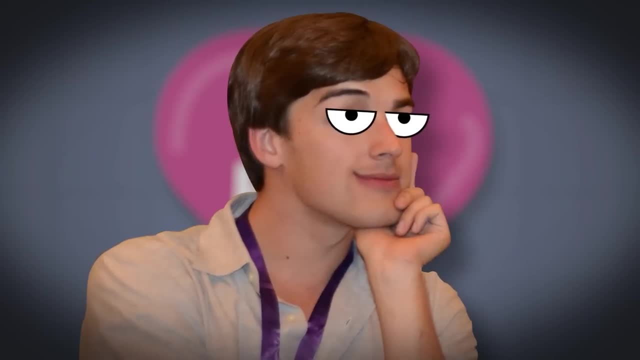 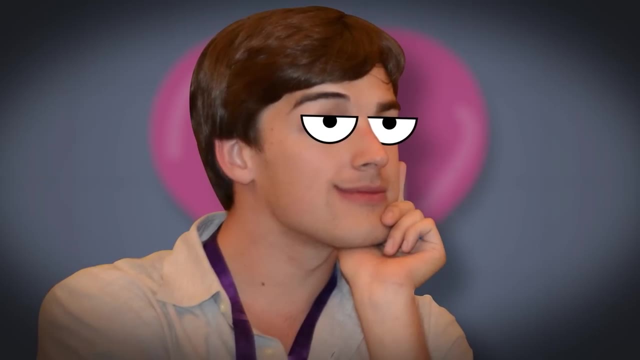 Be kind and respectful members of the community And Clown if you're watching- which you shouldn't be, since this is a theory video, but still, if you are just wanna say, take your time. There is absolutely zero pressure for you to make anything anytime soon. 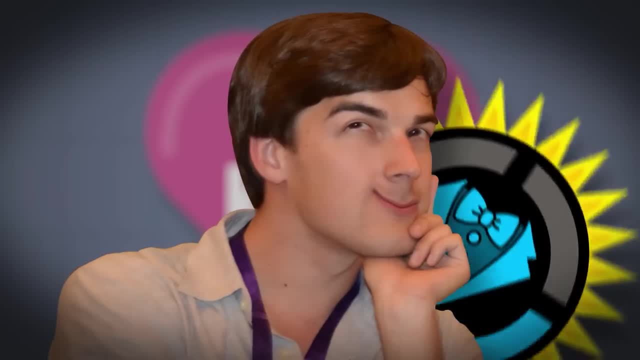 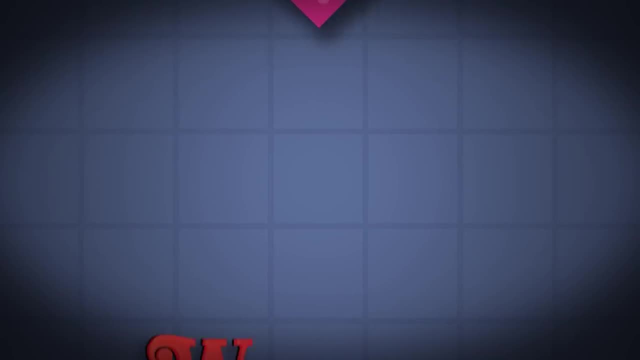 I mean, let's be honest, it took me seven years to finally launch style theory. Creating something cool takes time. One creator to another, just keep doing what you're doing and put your own mental health first. Alright, so with all of us on the same page, let's actually look at some of the clues that I mentioned earlier. 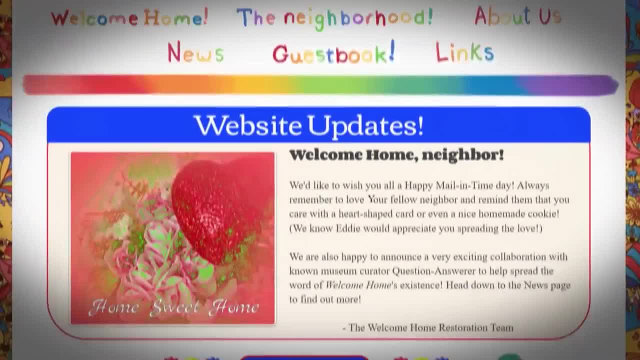 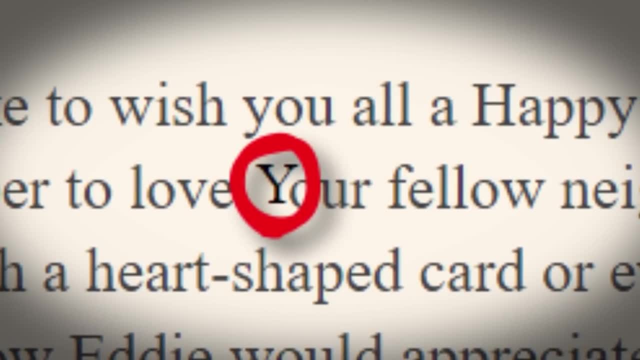 When you visit the homepage, you'll find Wall-E sitting on a rock, And below him is a newsletter explaining the latest updates. However, if you look closely, you'll see something that's quite literally out of place. The letter Y in the word your is sitting much higher than the rest of the text. 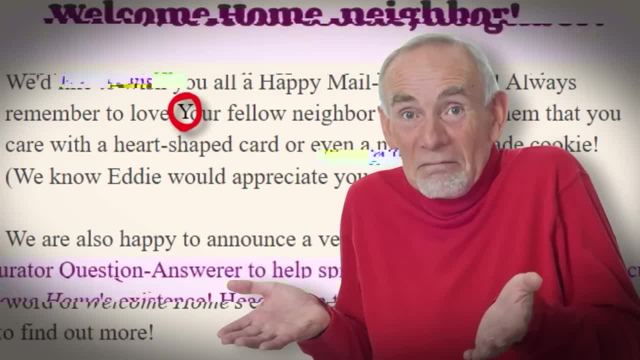 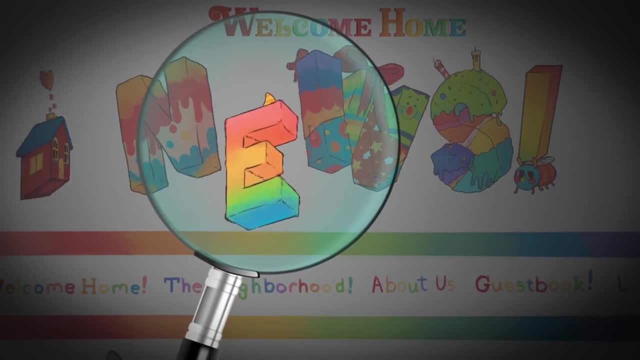 Now you might think that this is just a website glitch, Something that the creator didn't realize was there, But when you look through the rest of the site, you find the same thing happening over and over again: One misplaced letter on practically every main page. 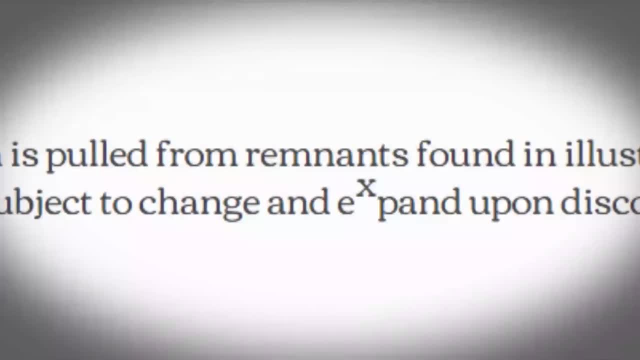 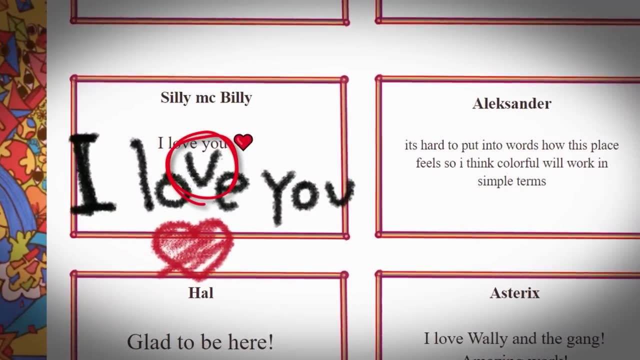 The W in Wall-E on the welcome home page is slightly too low. There's an X in the word expand on the neighborhood page, An O in the title of the about us page, An E in the news logo And a V in the I love you message over in the guest book. 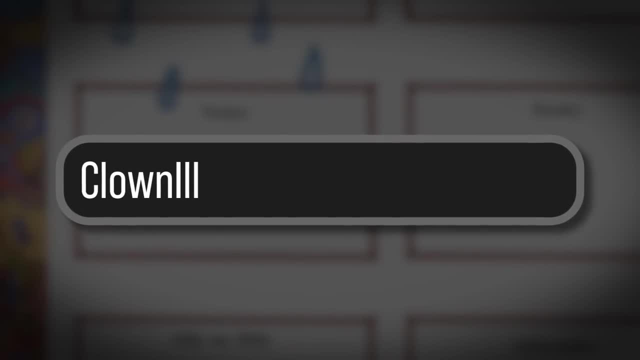 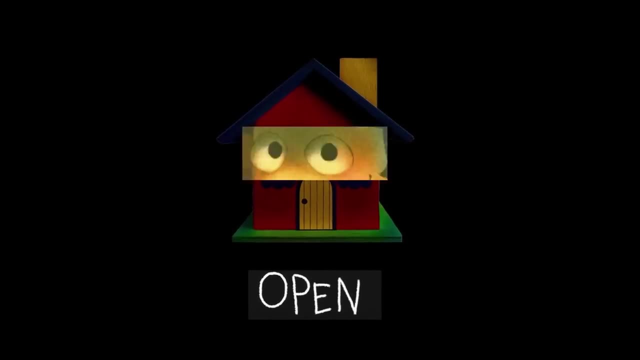 What do you do with all these letters? Well, you go back up to the URL bar and type in clownillustrationcom, slash, and then the letters YWXOEV. That then brings you to a brand new page that contains the image of a house with a gif of eyes over top. 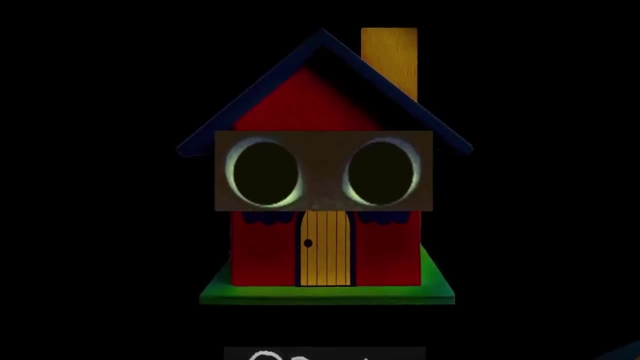 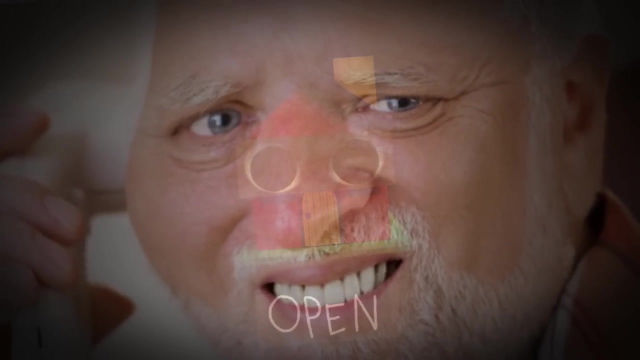 These eyes appear to be that of our lead character, Wall-E. Eventually, the gif stops showing only an image of his eyes, wide open, with dilated pupils, staring right at us, Which, I gotta say, is making me all sorts of uncomfortable. but this isn't the only secret that those letters unlock. 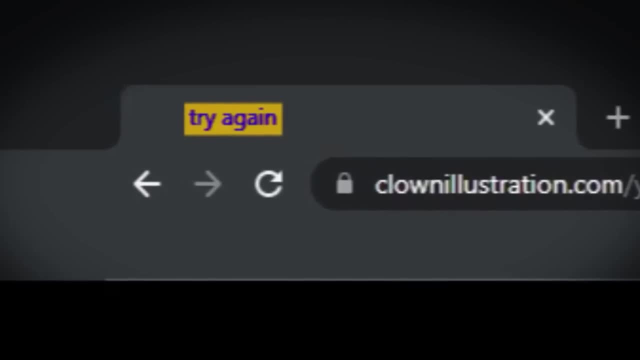 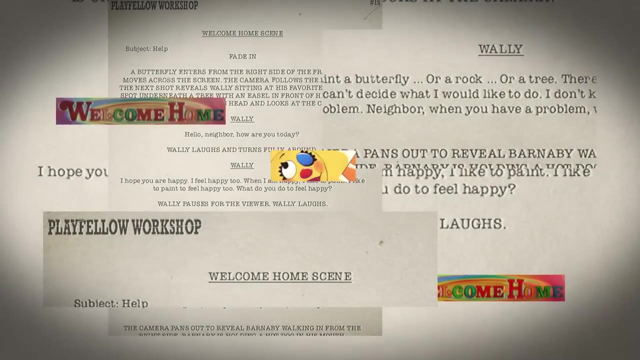 Notice the title tab of the website. here It says: try again. Clearly there are right and wrong combinations of all these letters. By putting in W-O-X-Y-V-E we get to see a page of the show's script. 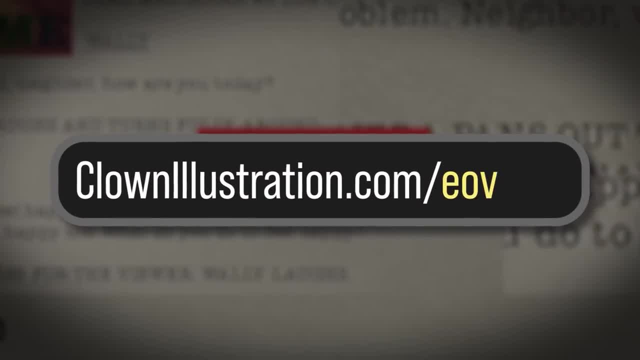 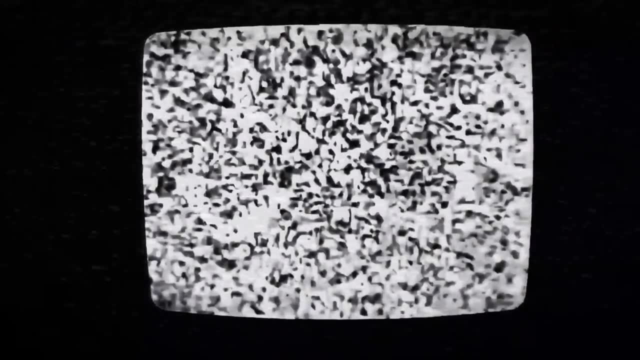 along with a gif that shows Wall-E's eyes looking at us, And if you try E-O-V-W-X-Y, you'll see a video of a TV screen with static. But when the 40 second mark hits, suddenly there's a flash of those same eyes staring at us through the screen. 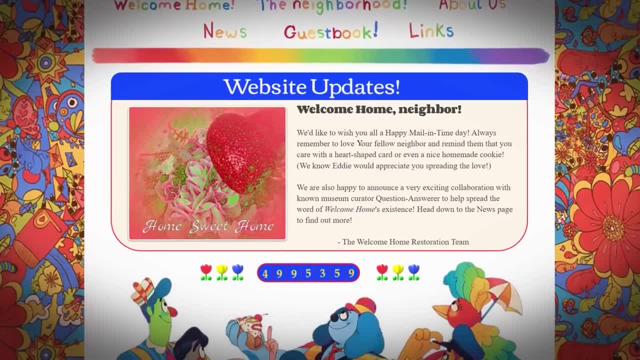 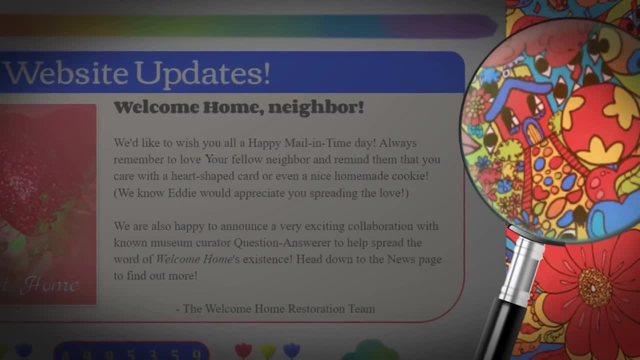 Something tells me we're being watched, And it's at this moment that you notice the designs at the edges of the website. What initially seems like loud flower power style designs of the 60s are actually a mass of eyes constantly watching us as we scroll through the website. 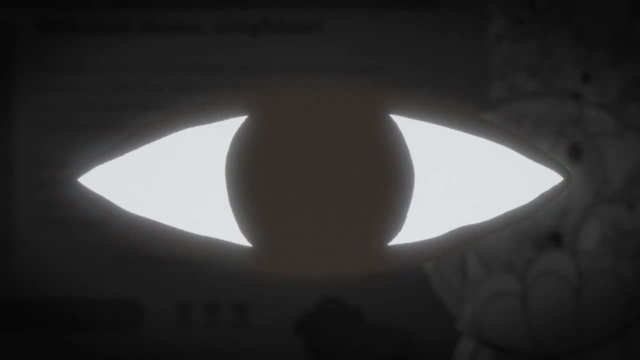 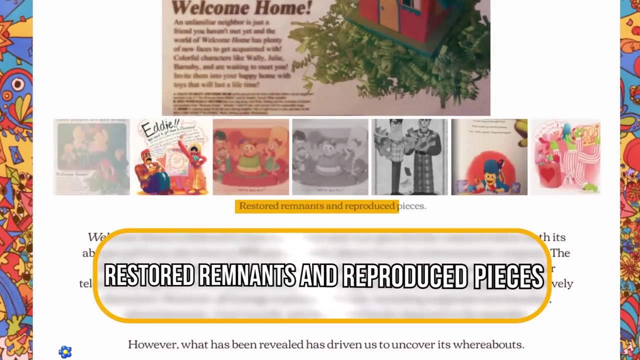 the various pages, But this doesn't end with it just watching us. Whatever this thing is, it's also trying to communicate with us. On the welcome home page, we find lots of images that are noted as being restored remnants and reproduced pieces. 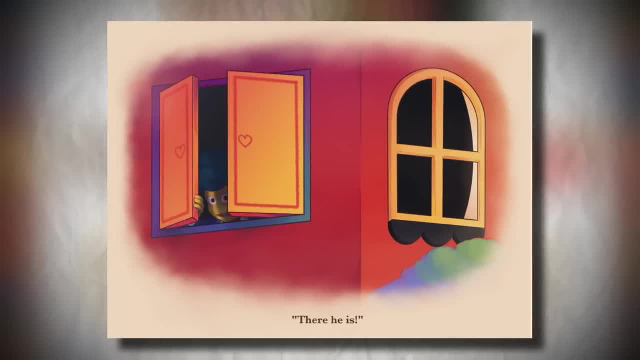 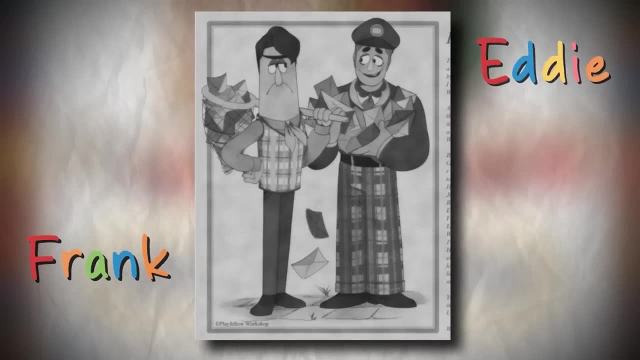 This is where we find that creepy image of Wall-E closing his window shutters. But there's also another image that's of interest here. There's what appears to be a newspaper clipping with a scene of the characters Frank and Eddie delivering mail. However, if you look closely, 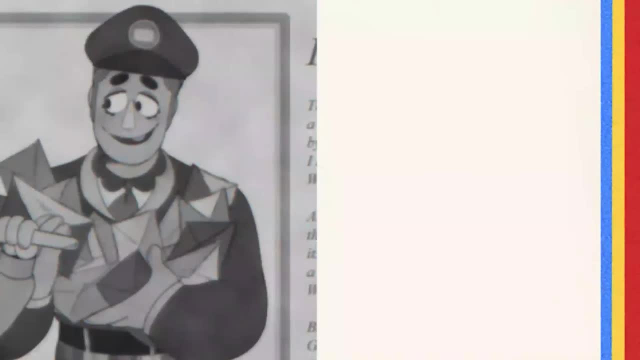 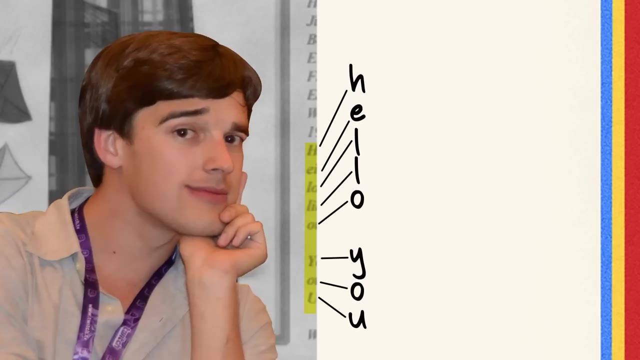 you'll see, part of the article is visible on the right hand side. Take an even closer look and you'll notice at the bottom. the first letters of each line spell out something: Hello, you Ha ha. Uh, that's ominous. 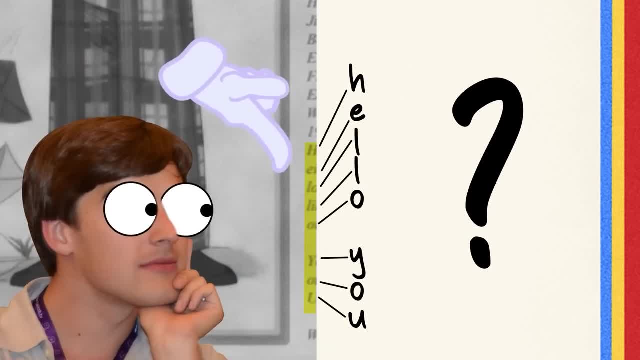 Who's speaking to us exactly. It's also not the only time that we see messages like this either. If you head on over to the about us page- the page where we learn about the recreation efforts, we can see a picture of Frank's head mechanics. 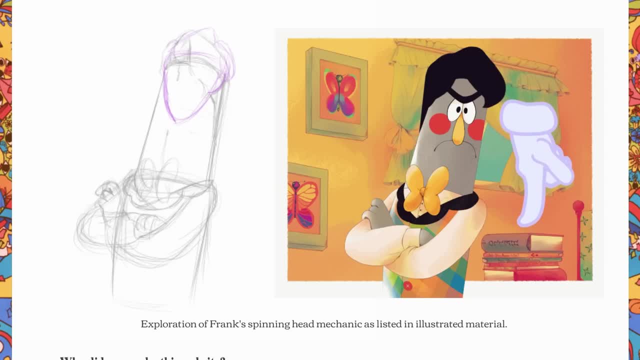 But in the corner of that image is a set of books, all with writing on the spine. The first couple are obvious and again give off that creepy vibe of something trying to communicate with us. Hello, it's you-know-who. 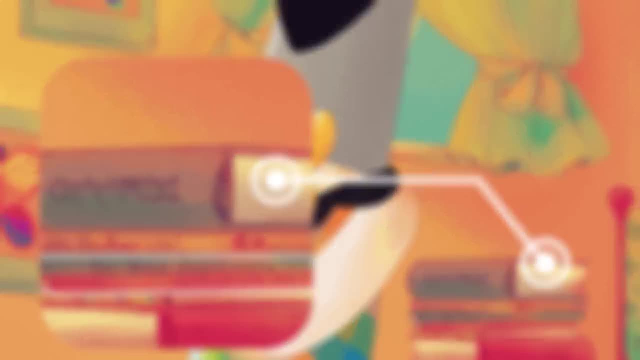 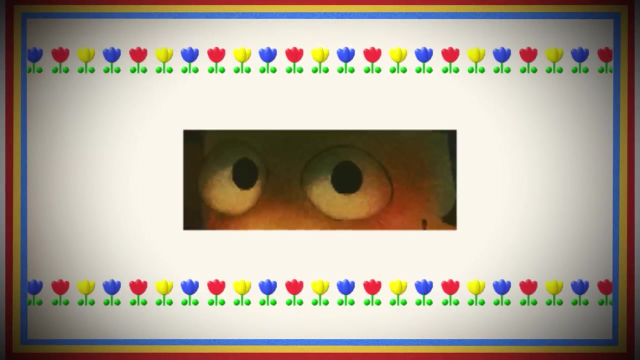 But it's the last books that really get into uncomfortable territory. They read: I'm your neighbor, Do you know about me? You do, I've seen you. So we know someone's watching us. We know they're trying to communicate with us. 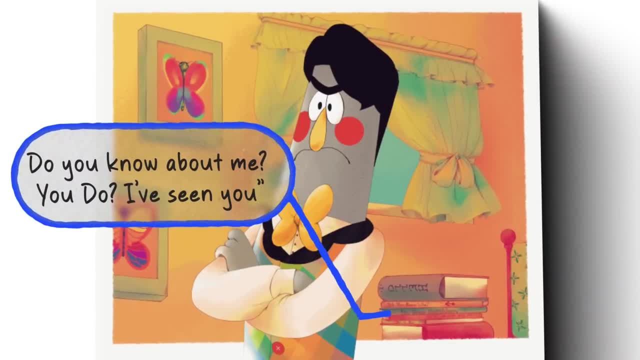 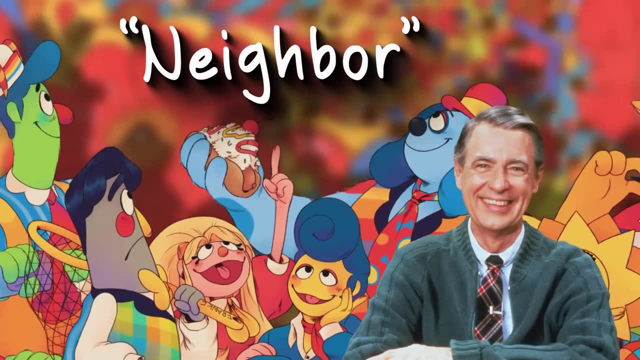 But who are they? They assume that we know them, So we should probably figure out. who's on the other side of those book spines. Feels very much like someone from the show in some way calling us neighbor. It's very Mr Rogers-esque. 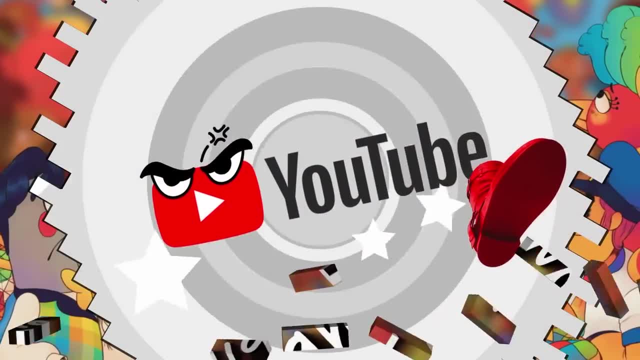 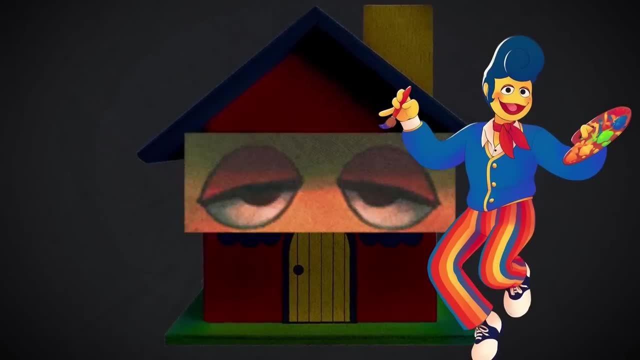 like a TV host addressing the people that are watching Brick-in-the-fourth-wall YouTube style. Could it be that the reason that we saw the eyes of Wally on those mysterious pages was because he's the one trying to communicate with us? Well, the only way to know for sure is to keep on searching. 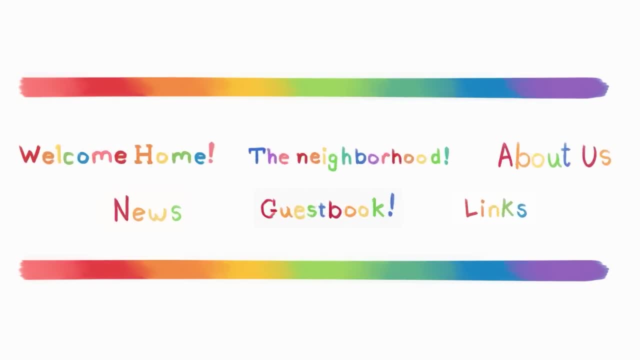 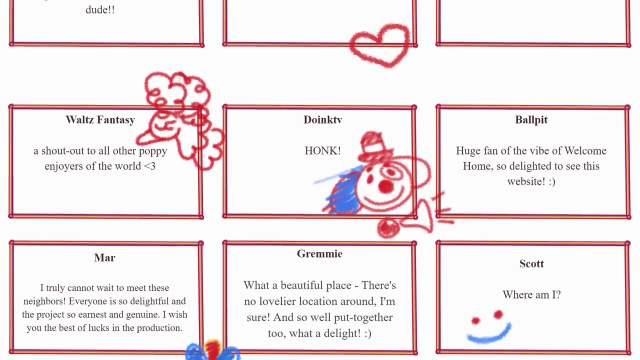 And I want to go all the way to the end, to the page that's filled with probably the most lore of this entire project: the guestbook. This guestbook is for people visiting the site to leave comments, but that's not the only thing the page displays. 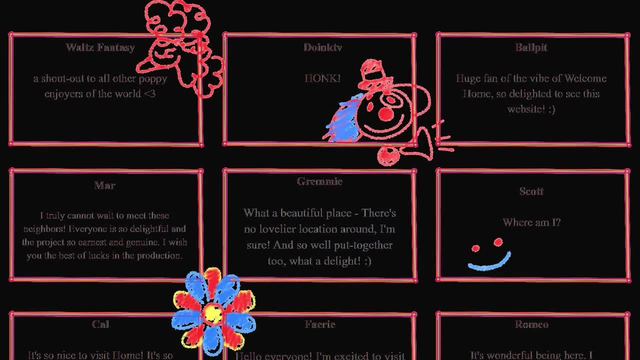 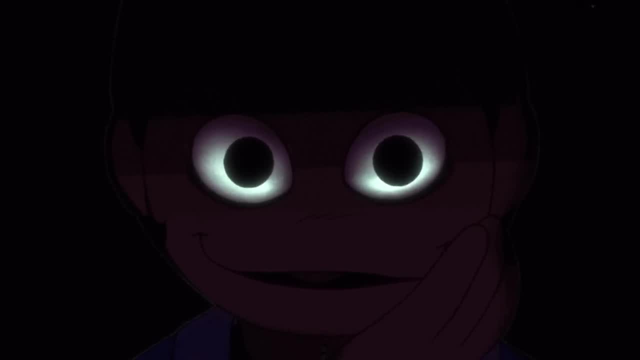 Sometimes there are drawings next to those comments which aren't made by regular users like you and me. Someone or something has drawn them on the page, Most likely the one who's been watching us this entire time, And this is where things start to get even cooler. 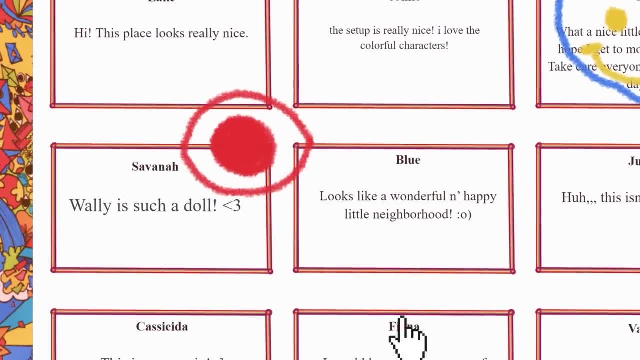 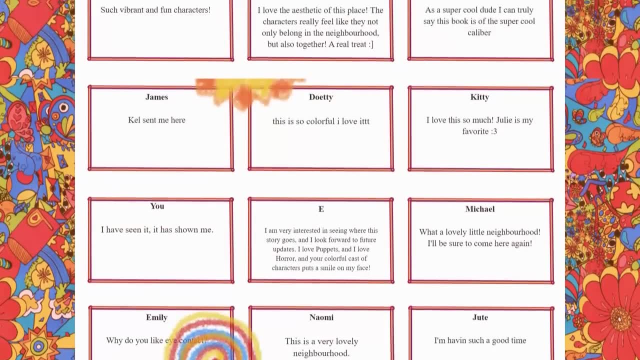 Sure, having even more pictures of eyeballs drawn next to comments is unsettling, but that's not all they're doing. If you open the image in a new tab, you'll find almost all of them have interesting file names. For example, on page three there's a spiral drawn in red, yellow and blue crayon. 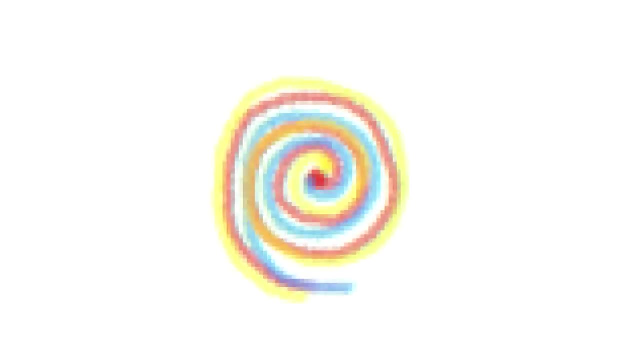 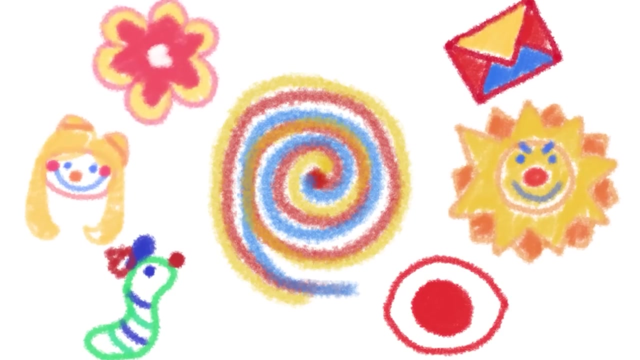 next to a comment that asks: Why do you like eye contact? And if you open that image up in a new tab, you find the response. So you will know I am looking at you, neighbor, I am talking to you. So whoever's drawn these images is definitely connected to everything else that's been going on around here. 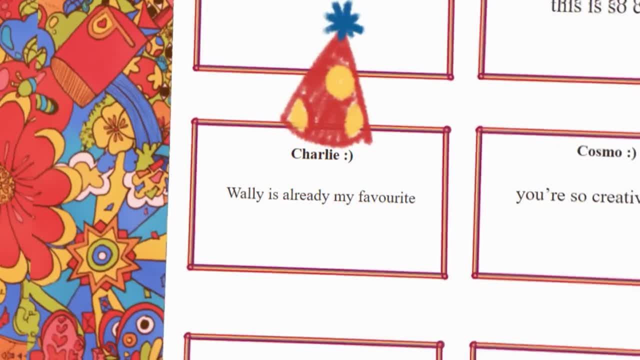 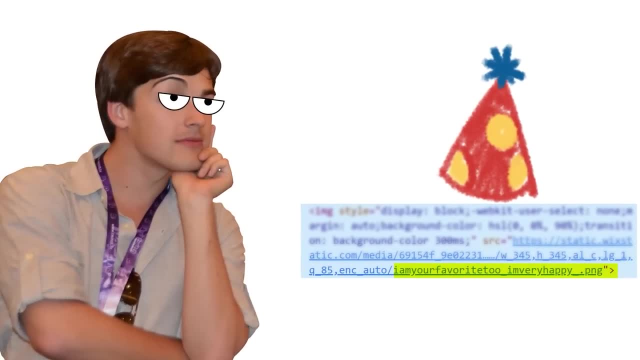 So who is it? Well, we get clues to that answer throughout the rest of the guestbook. For instance, there's one comment that says Wally's my favorite, To which the website draws: I am your favorite too. Awfully presumptuous of you there. mystery host. 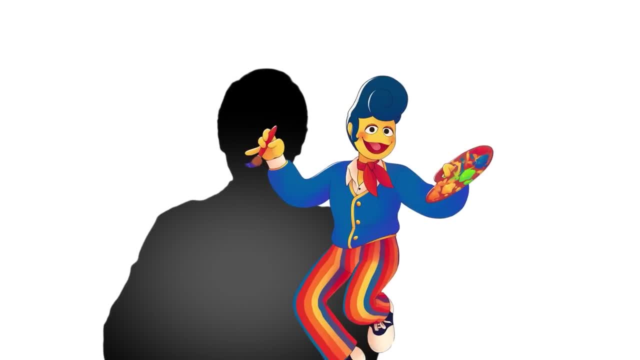 So we know that Wally and this character aren't one and the same, Except maybe they are In another comment. that says: I hope Wally knows that he's my favorite. the title tab says: I'm your favorite. That makes me happy. 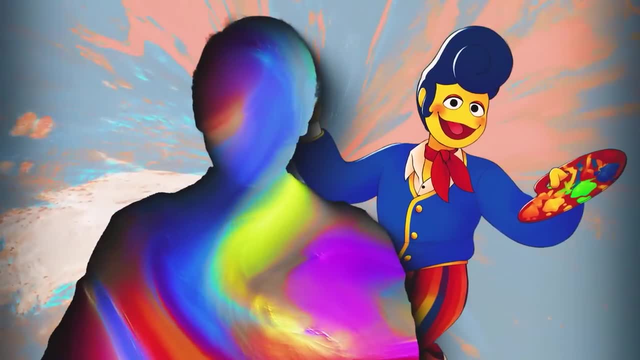 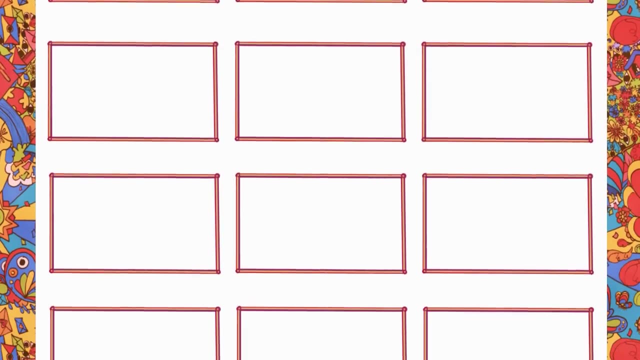 So are you or are you not, Wally? Well, it seems like the answer may actually be yes and no. When you go to the last page of the guestbook, you're presented with a lot of blank entries, Which I don't know about you, but feels awfully suspicious. 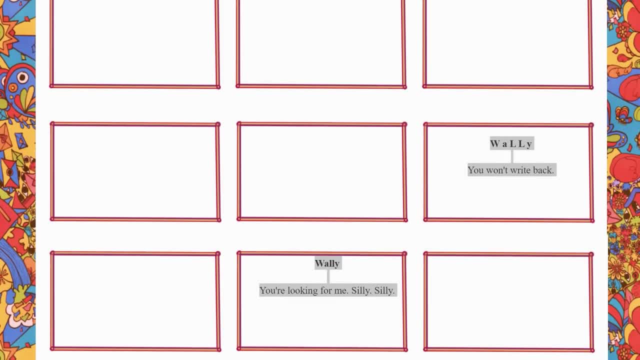 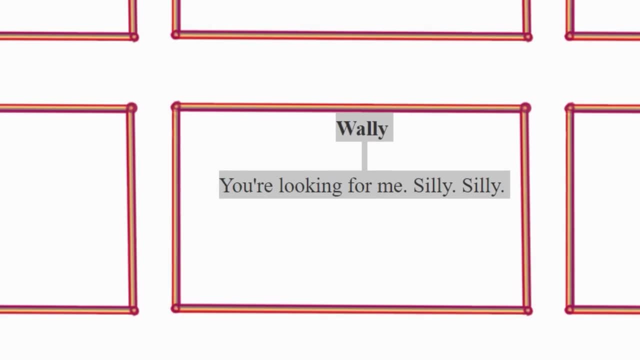 So if you hit select all in one of those empty guestbooks, it suddenly reveals that there's hidden text here from Wally That reads: You're looking for me, Silly, silly. But right next to it is another entry. 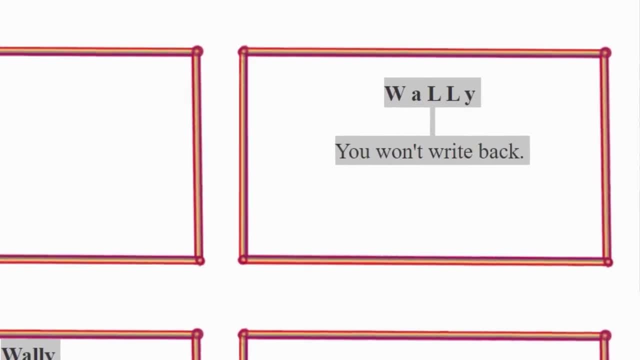 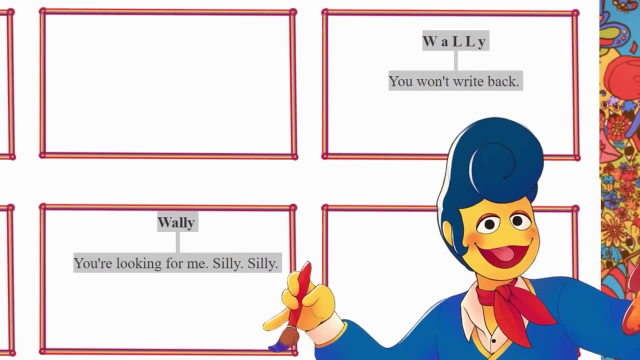 Also credited to Wally, except this time it's like somebody wrote his name and then put it through a Spongebob meme filter. It says You won't write back The fact that both of these are identifying as Wally, just with one of them corrupted. 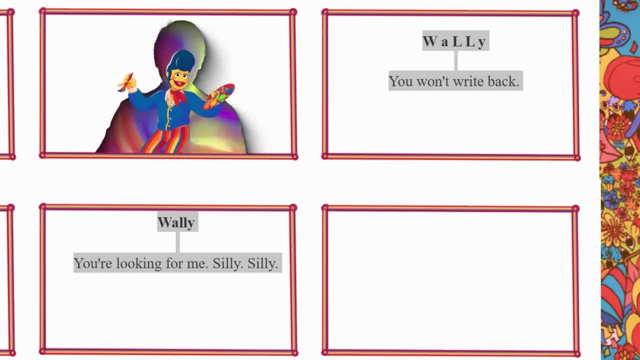 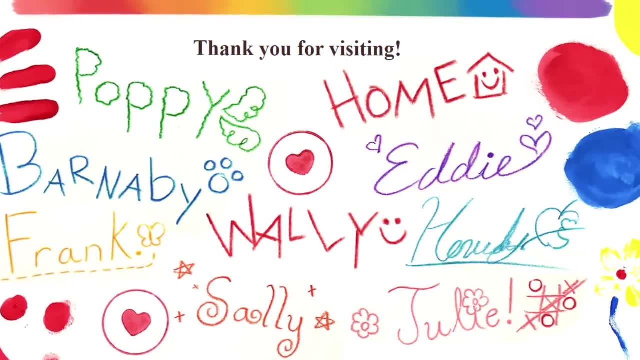 it seems to indicate that there are either two entities inside our beloved host or there are two Wallys running around, The real Wally and something else. But what? Well, at the bottom of each webpage, all the characters sign their name. 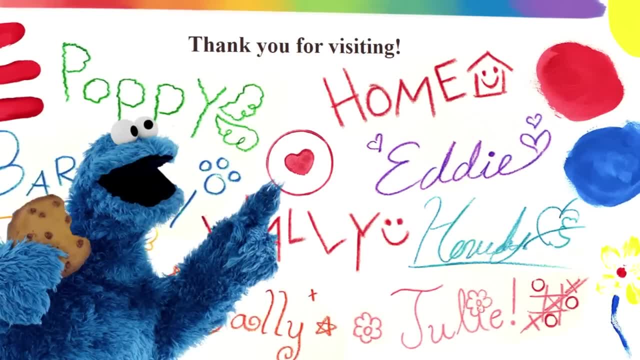 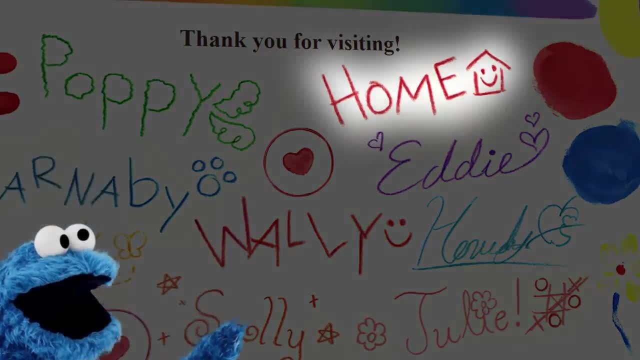 Each with a unique signature. But, to borrow a phrase from a rival kids show, One of these things is not like the other, Or should I say, two of these things are actually exactly like the other. Notice how the writing for home is the same as the handwriting for Wally. 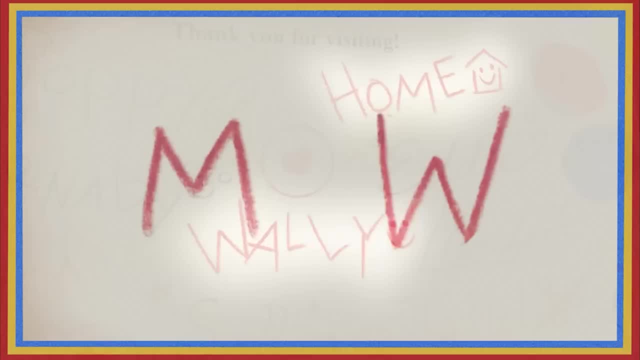 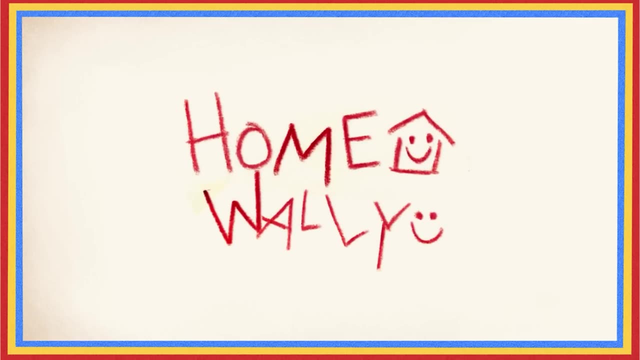 Same red crayon, same style of writing, especially when you compare the M and the W. Wally and home are connected in some way. They seem to be one and the same. This is also heavily supported by another one of the guestbook pages. 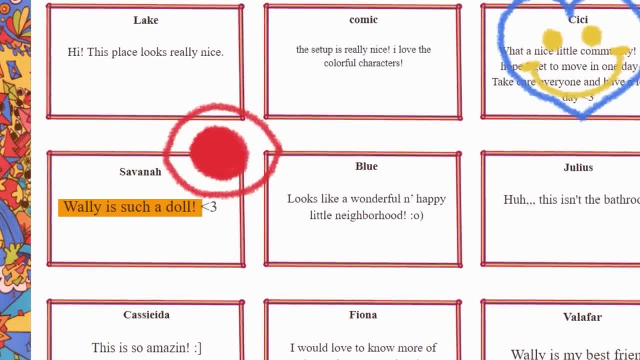 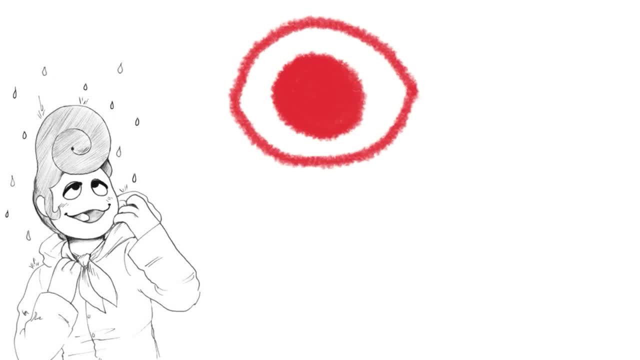 On page five it says that Wally is such a doll And the website's response is a picture of an eye titled No, a puppet. It's a double meaning. Not only is Wally the character, a physical puppet, but he seems to be getting puppeteered by something else behind the scenes pulling the strings. 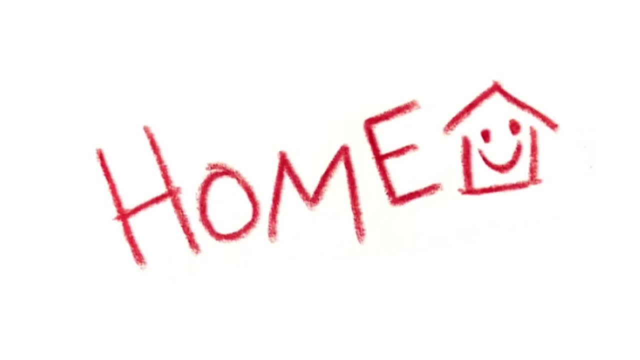 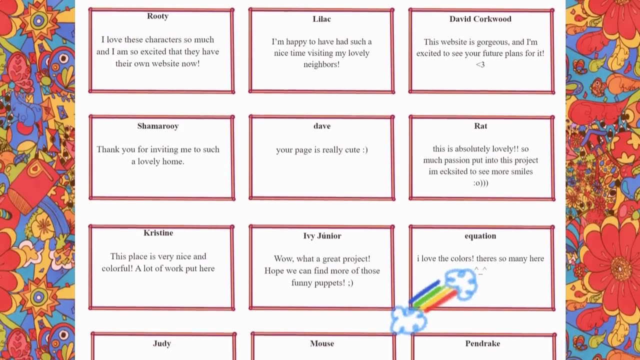 Whoever or whatever home is supposed to be. There are a lot of other messages hidden throughout the guestbook and I'd encourage you to go and check them out, But I figured I'd try somewhere else to see if it would yield different results. 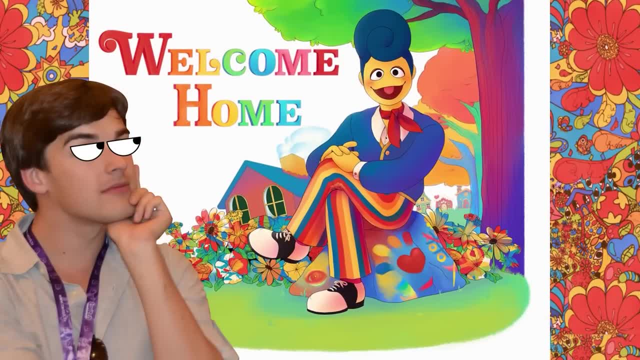 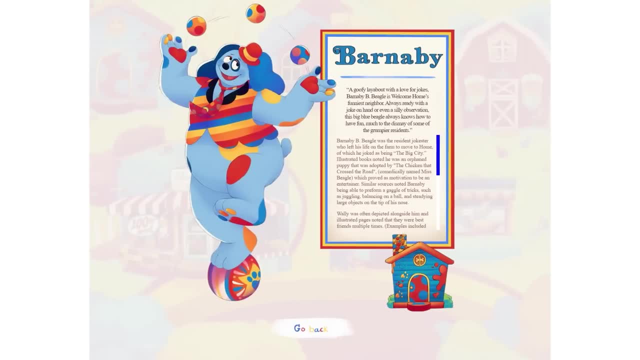 And lo and behold, my hunch was correct. This site is hiding a ton of information in very unique places. On the The Neighborhood page, you can actually click on the houses to learn about each of the characters. Each one gets themselves an illustration. 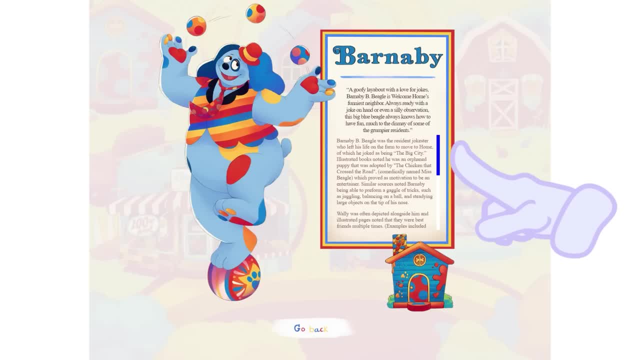 and then a page on the right with their key character traits. However, if you do what I tend to do with these types of mysteries and just click on everything in sight in the hopes of finding clues, you'll actually be rewarded If you happen to click on the word. 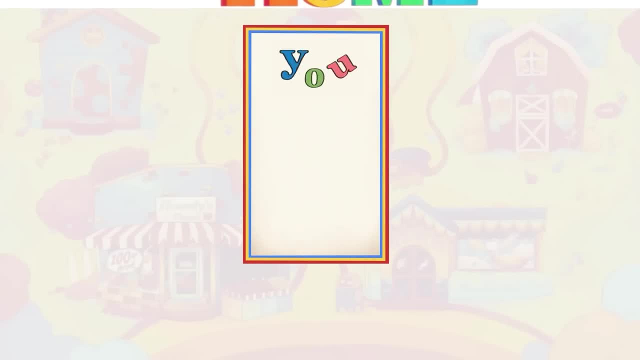 You and the word You're at the top of the page. you'll be taken to a brand new screen, One that has a description card like all the other characters, only this time it has you- Yes, you, The one watching. 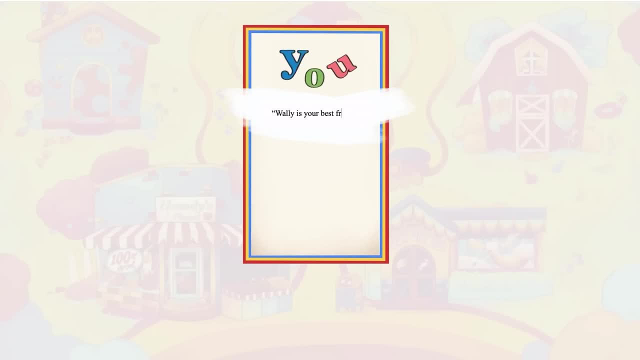 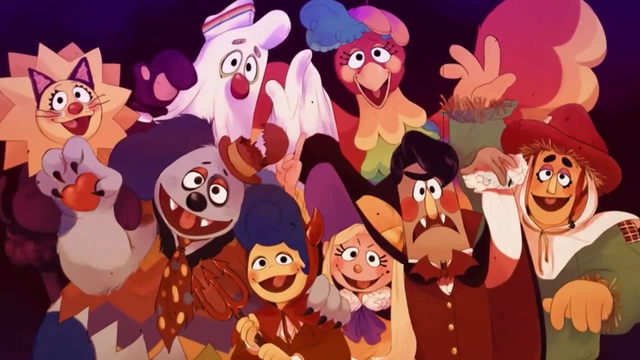 And you got yourself a single line in your description. Wally is your best friend, So that, along with the constant calling of people in the guestbook Neighbor, it's kind of giving me vibes of a cult where everyone refers to each other as brothers and sisters. 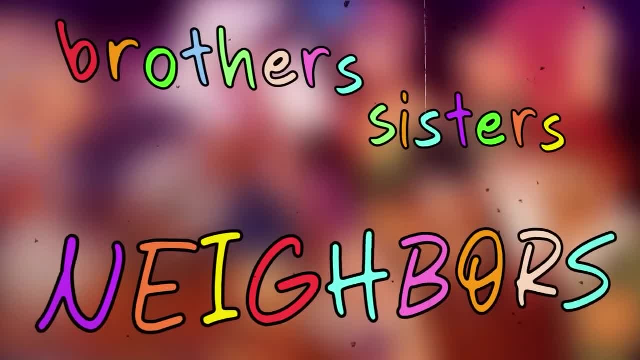 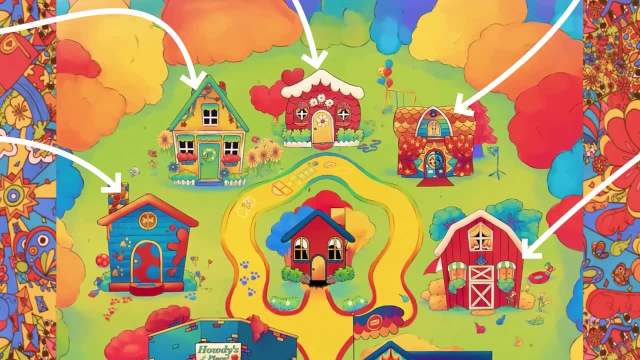 or in this case neighbors, rather than by their actual names. Speaking of weird details in the character descriptions, all of these characters, minus Wally, don't originate from home. They all moved here from somewhere else. They all have friends and family. 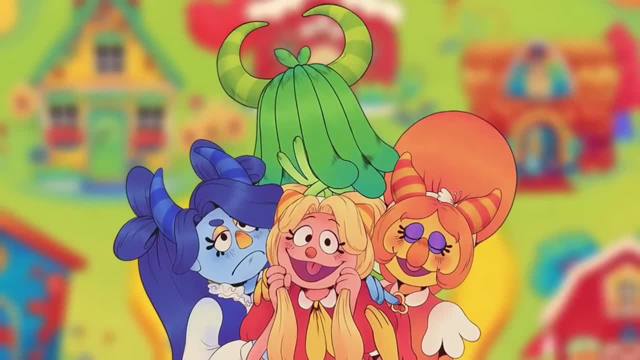 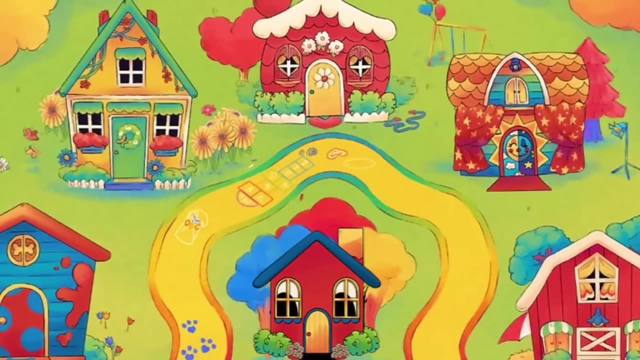 We even see a picture of Julie and her siblings elsewhere on the site, but they don't exist inside of home, Which again gives me some creepy cult vibes where members are encouraged to abandon their former lives and move to live with other cult members in a closed off community. 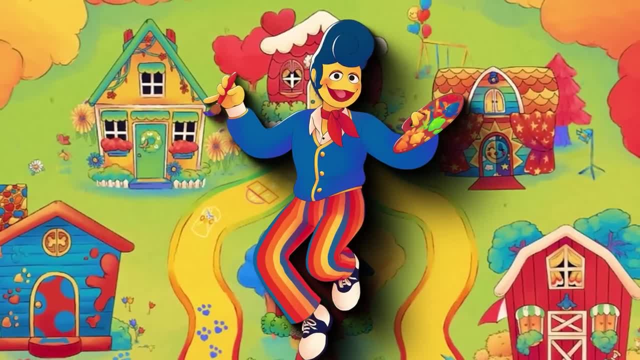 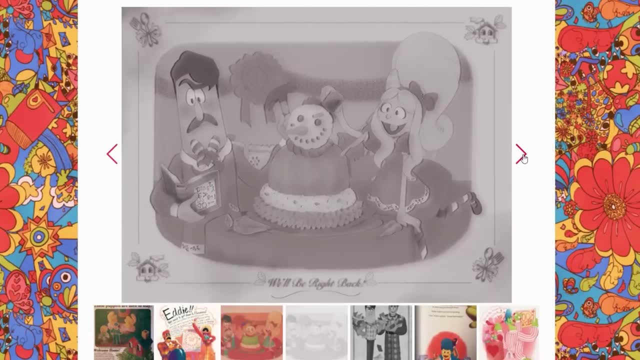 And, given that Wally is the one that never had to move, my gut's telling me that he's the one in charge, And my gut seems to be right. As I looked through more and more of the images on the welcome page, I noticed one very specific and tiny detail. 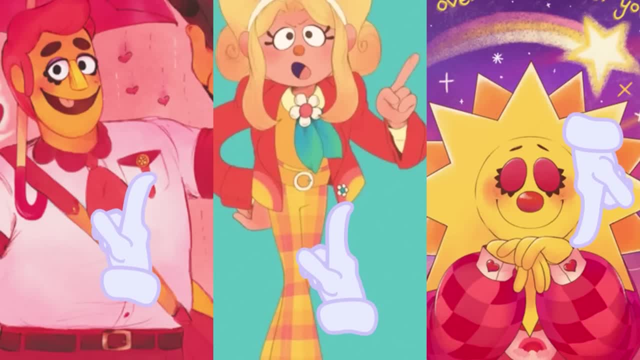 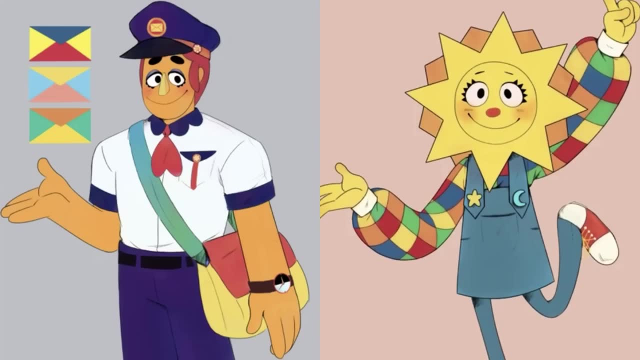 The characters all wear badges, pins or cufflinks related to their personality and traits. Some are pretty darn obvious: Eddie has a male pin on his hat because he's a mailman. Sally has a star and moon pin on her because she is literally a star. 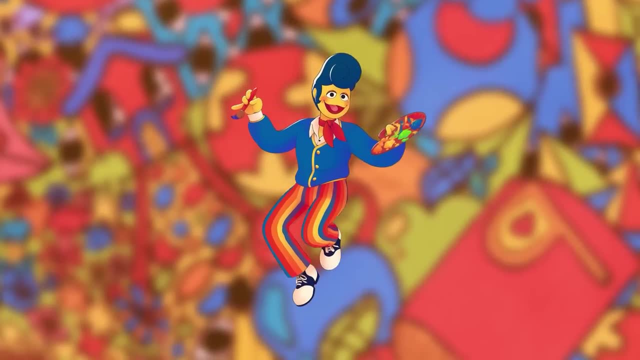 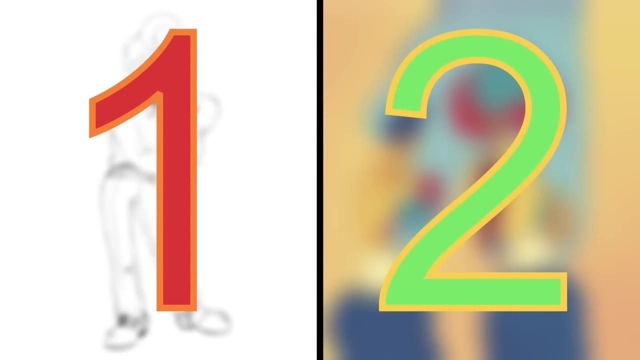 But what about dear old Wally? I expected to see him with some kind of art base- pin, paintbrush, easel, crayon- But those were nowhere to be found. Instead, there are two images on the website that show what cufflinks Wally's wearing. 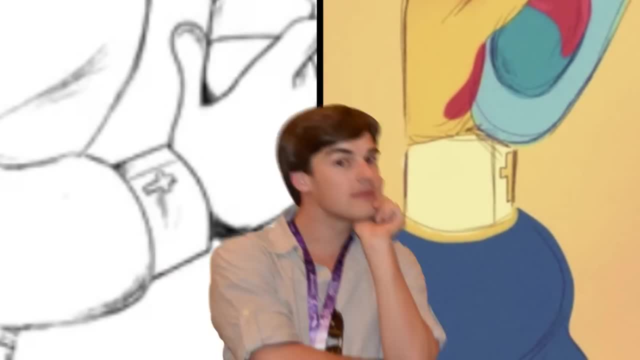 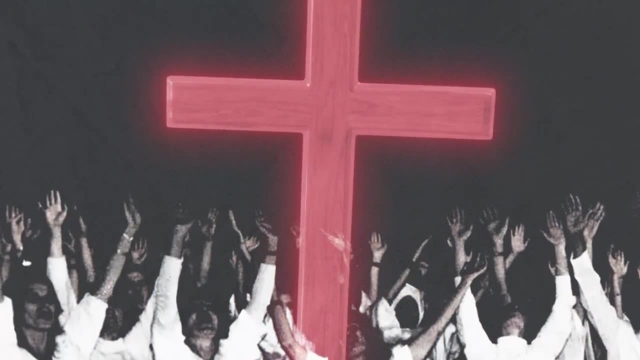 and they're pretty surprising. He's wearing crosses, Which doesn't really feel all that thematic for a character who's a painter. Instead, that's the sort of thing that you get out of a religious leader: A vibe that starts to get even stronger if you go back to the earliest days of the website. 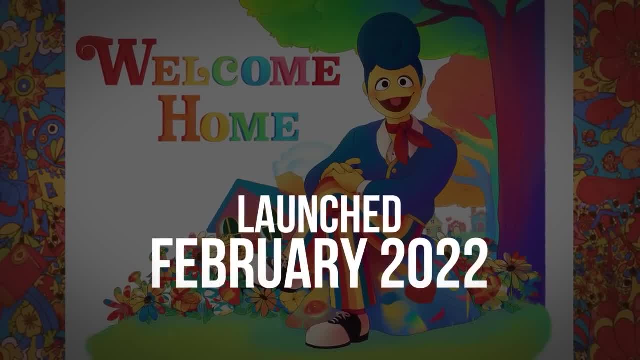 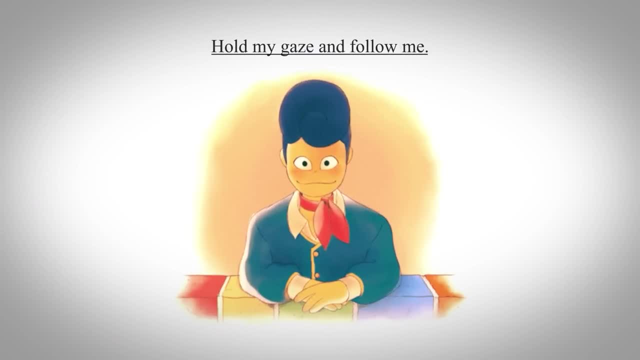 Now, this website was first launched back in February of 2022. And back then it looked very different than it does today. At one point, there was this image of Wally staring directly at us With a simple phrase above his head. 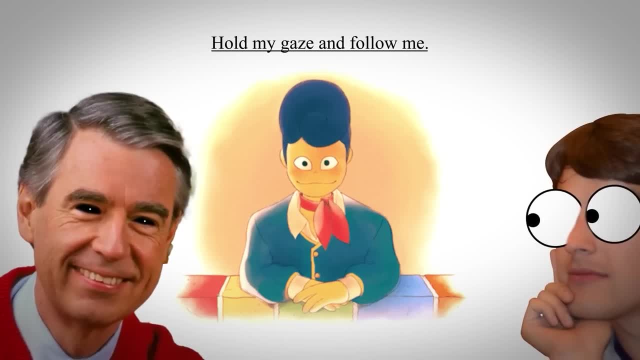 Hold my gaze and follow me. I don't know about you, but if Mr Rogers started speaking to me that way, I'd be catching the first trolley on out of here. No, this sort of phrasing is very similar to the style of speech used by religious figures. 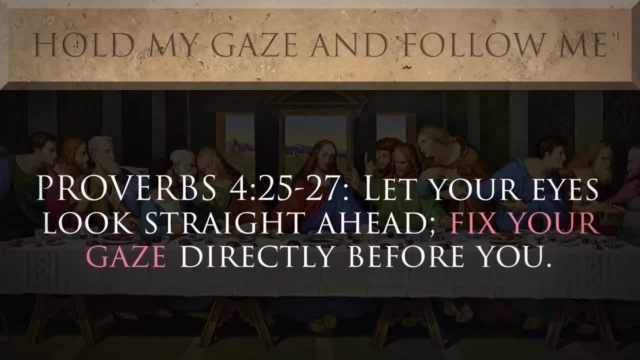 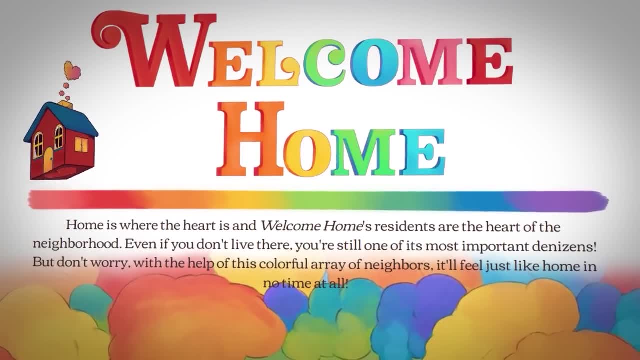 Especially Jesus, from various passages throughout the Bible where he would ask his disciples to follow him. It's also a tactic used by cult leaders as they indoctrinate new members. But bringing it all back around to the current website, if you visit that neighborhood page that I mentioned earlier, 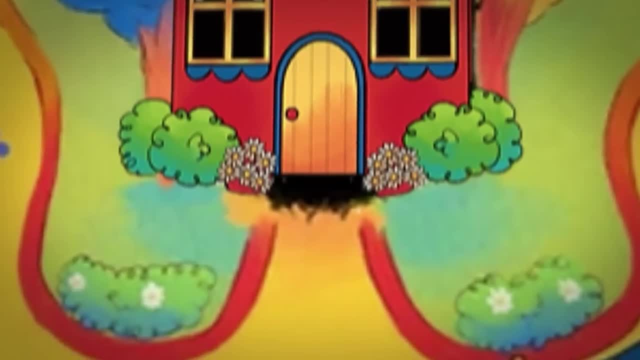 and take an even closer look, you might notice that Wally's house has this pulsating black goo coming out, And with internet projects like these, we all know that black goo is never a good sign. To my surprise, that space below the house was clickable. 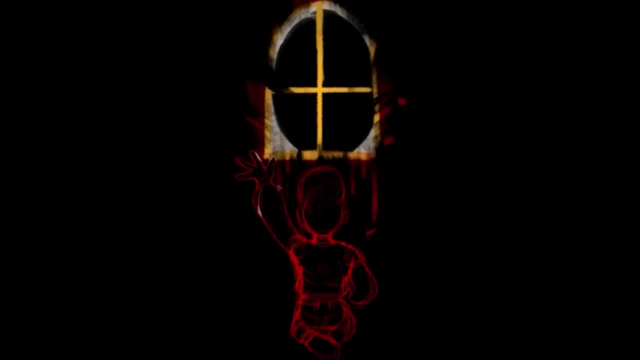 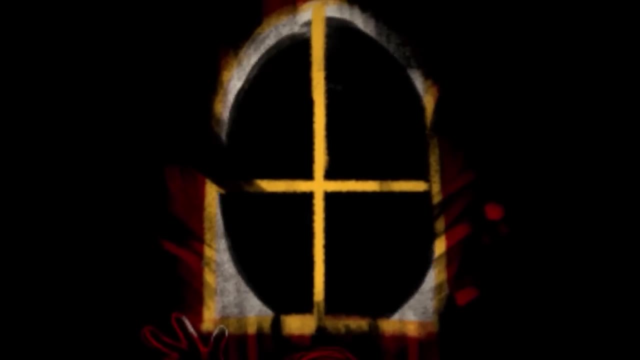 So I clicked it and I got this: A black image of Wally drawn in red, kneeling before the eye of his house with one hand raised. I mean, this is the most creepy thing that we've come across so far. And it gets even creepier because the title tab text is listed as: 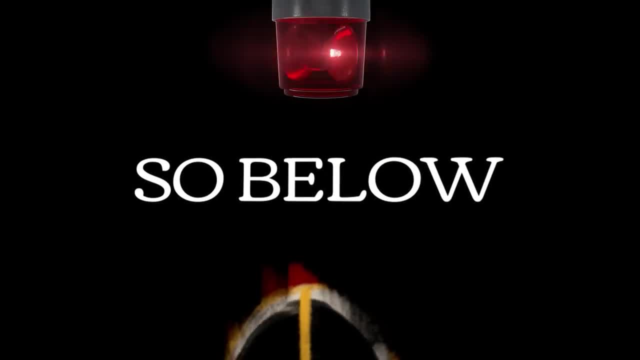 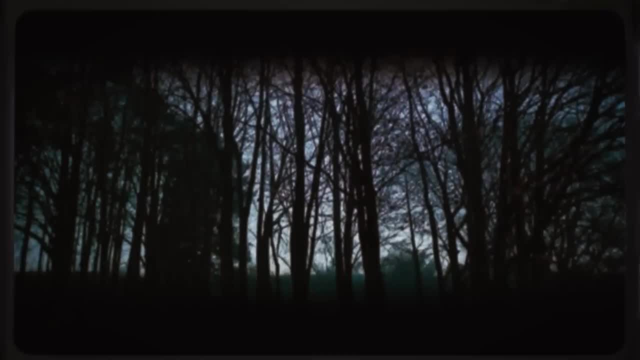 So Below. If those two words don't immediately ring alarm bells for you, that's fine. To me, though, as someone who's done his fair share of weird internet research, that phrase always leads to one thing: It's actually half of a phrase that you see a lot. 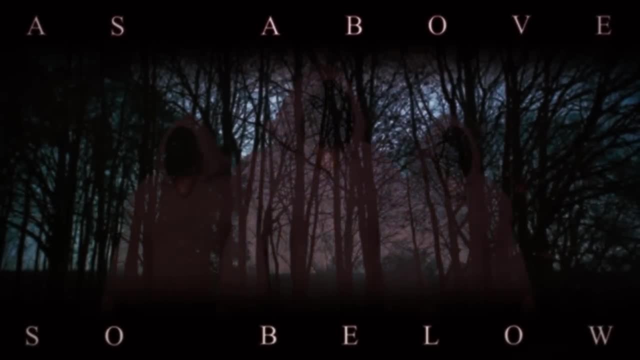 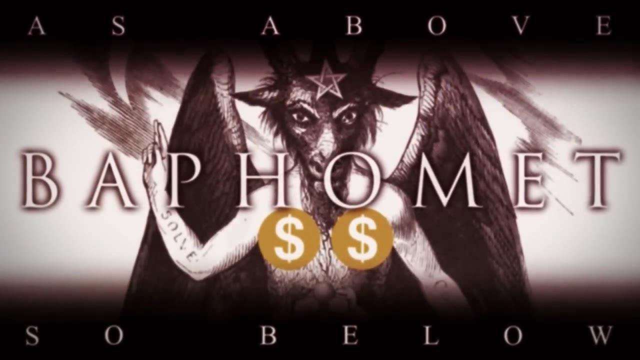 As above, so below, A phrase that's usually used in conjunction with occult practices, Not just any practices either. More often than not, the phrase is associated with one particular image of the deity Baphomet. Baphomet was worshipped as a deity by groups like the Knights Templar. 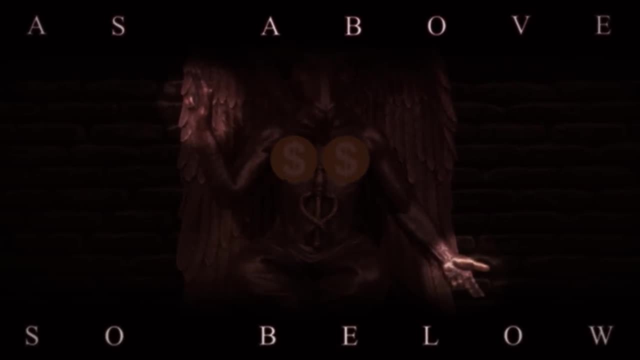 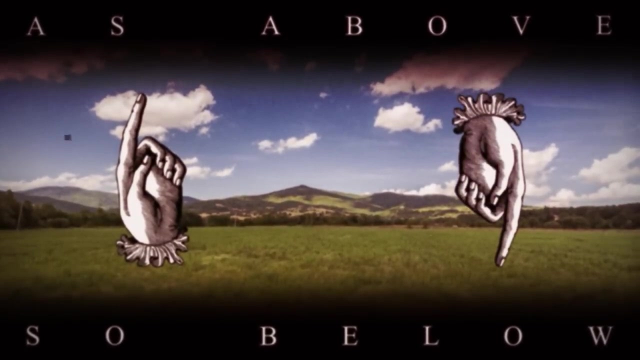 and represented balance, with the two finger salutes pointing up and down. Hence, as above so below, It's a symbol of mercy and justice, As well as explaining the idea that if things are a certain way in the heavens, so shall they be down below. 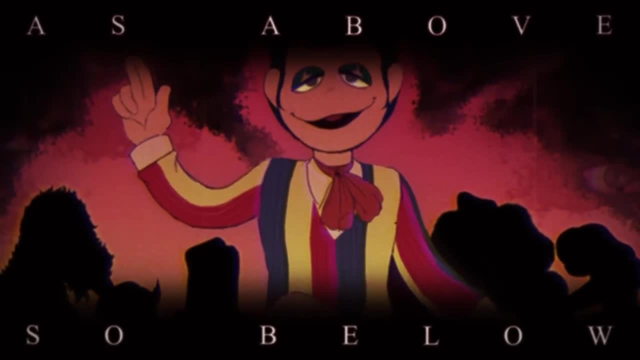 And here on Earth. And, fun fact, if you take a look at Clown's professional art page, there's actually an image of Wall-E pulling the exact same pose. Now, it's at this point that I should probably mention that all the stuff on that particular website. 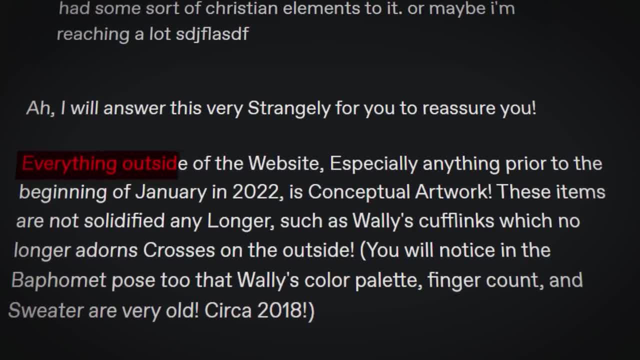 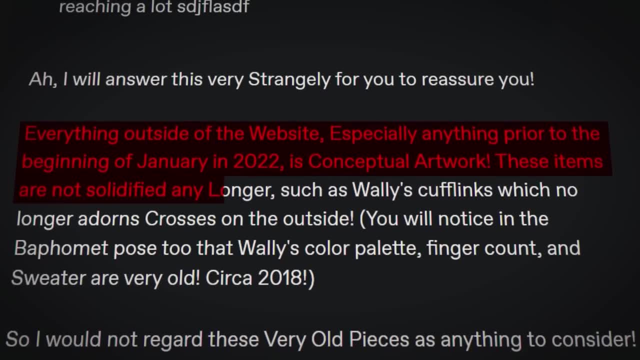 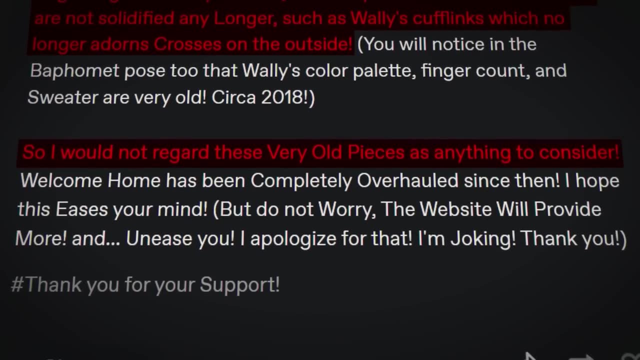 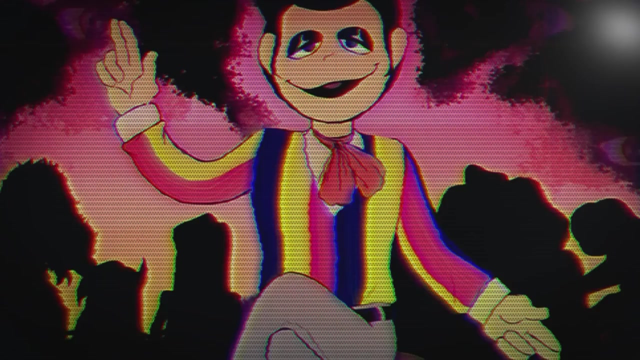 isn't considered canon by Clown Quote, So that Baphomet image is definitely not canon. but it does seem like some of these ideas have persevered throughout the various updates of the website. Hence that other image still being titled so below, despite various website updates. 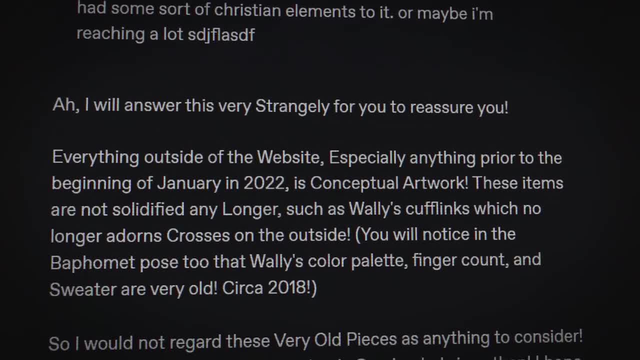 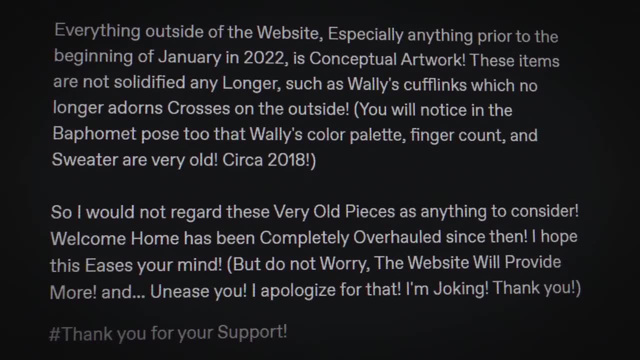 I've also seen comments saying that this statement disproves any sort of religious or occult theory. but looking at these words from Clown, which are the only comments that I could find related to this particular topic, I don't think that's actually what they're saying. So back to as above so below. Baphomet wasn't only depicted in that one pose. He was also regularly depicted with children surrounding him. because the idea was that children wouldn't immediately see him as the devil, They should be allowed to make their own decisions, rather than being told how to interpret something. 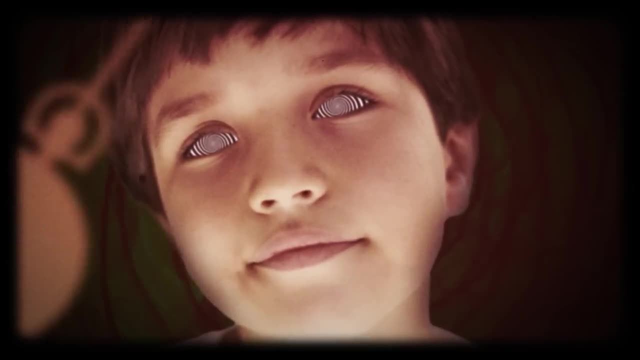 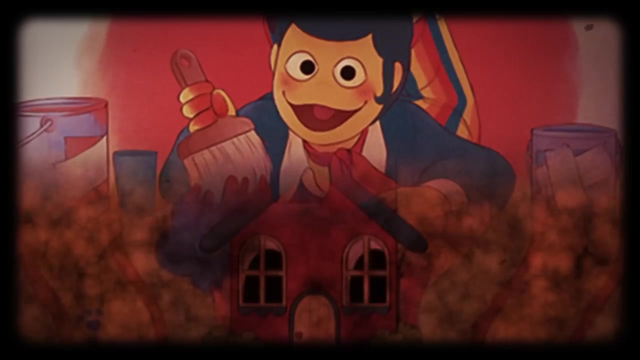 Specifically, the worshippers of Baphomet were against the indoctrination of children, which is pretty darn interesting if Wall-E is now fulfilling the role as some sort of puppet deity. In short, all of this seems to imply that, just like Baphomet represented balance, 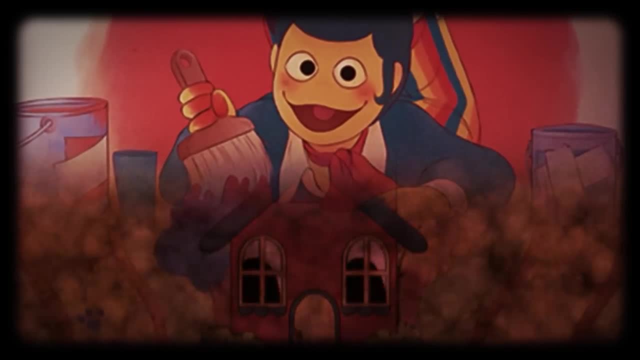 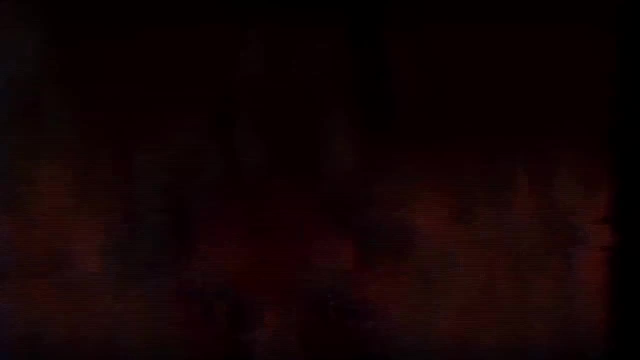 Wall-E and Home also balance each other out. Wall-E is the friendly childhood host and Home is the darkly chaotic, perhaps even evil, monster. On the About Us page we see some of the artwork that's being received from an anonymous source. 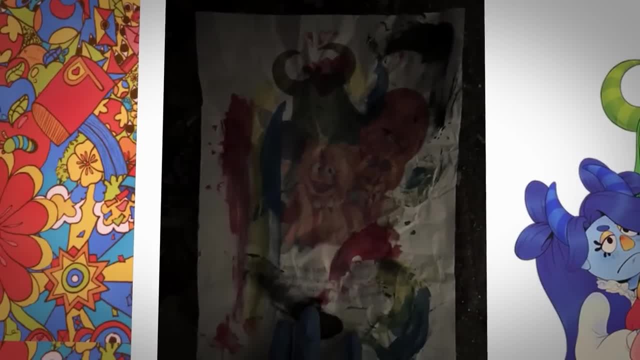 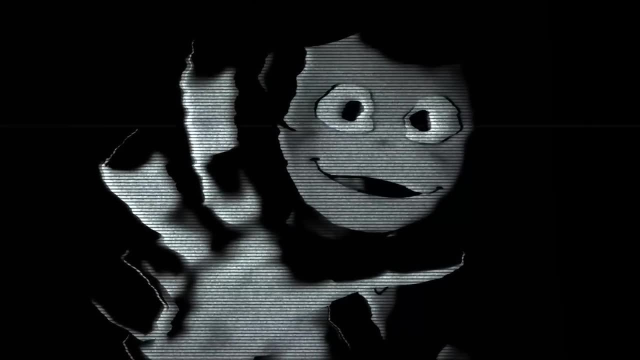 but the original artwork always arrives in a damaged state, covered in red, yellow and blue paint, The colors that Wall-E uses, Again showing us that this isn't just a show, but that the real puppet of Wall-E is alive and purposely trying to reach out to us. 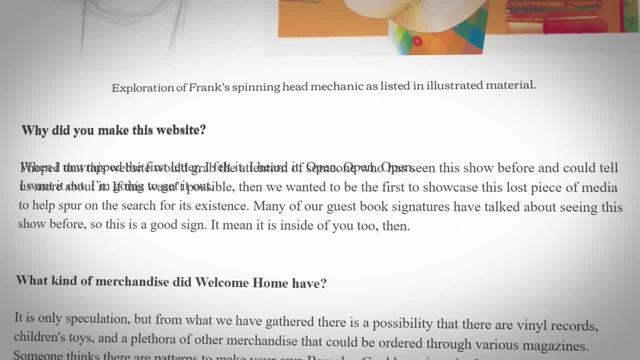 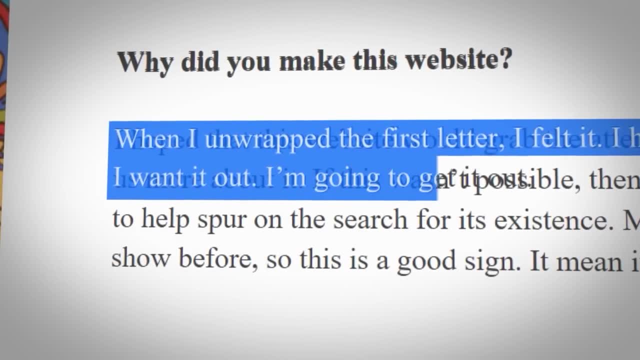 On that same page there's an FAQ section where there's some text that overlaps, Text that reads: When I unwrapped the first letter, I felt it. I heard it: Open, Open, Open. I want it out. I'm going to get it out. 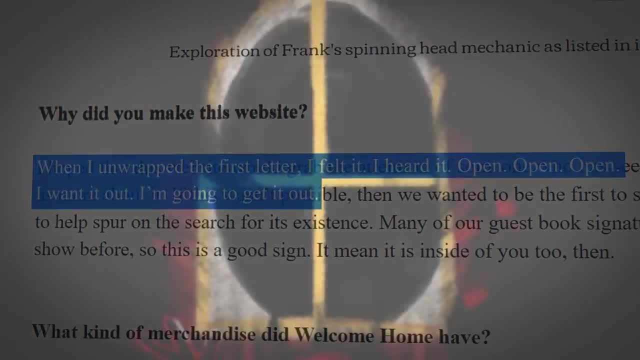 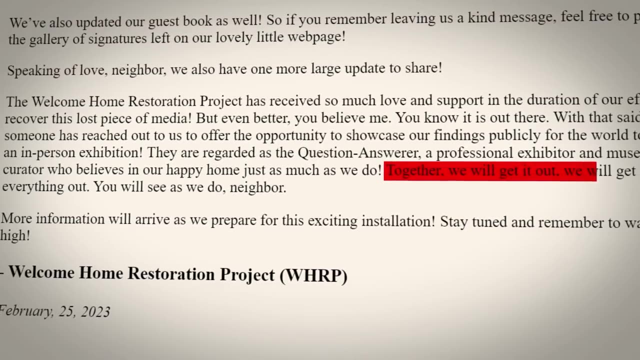 What does he mean? get it out? Are you talking about Home? We see the same type of language on the news page, where we're told that a museum curator is wanting to put on an exhibition for all these findings Together. we will get it out. We will get everything out. 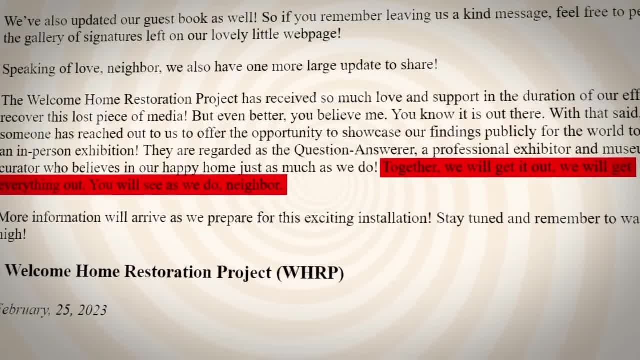 You will see, as we do, neighbor Now, that right there, that sounds like indoctrination at its finest, Wall-E has managed to brainwash these people. Now, thanks to this exhibition, they're going to be able to spread the word of this show. 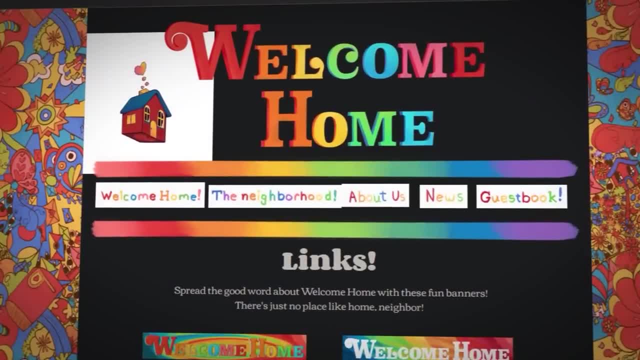 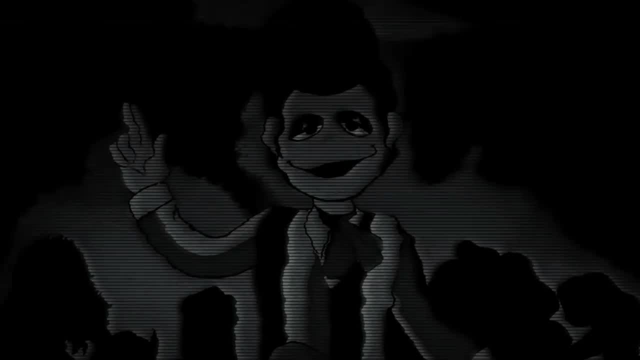 this cult to the masses. The links page, for instance, is literally labeled as: Spread the Good Word- The Doctrine of Wall-E. But what exactly is Wall-E's doctrine On the surface, thanks to that Baphomet imagery? 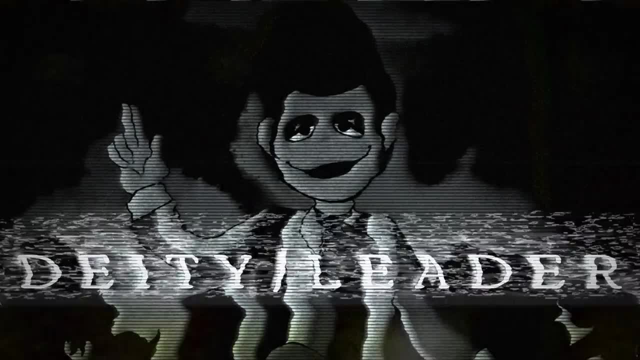 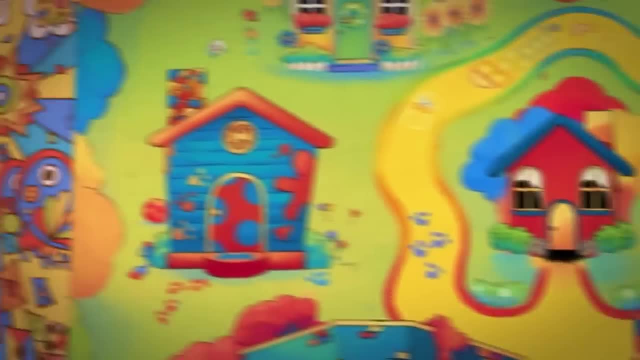 you might think that Wall-E is both a deity and leader, but I don't think that's the case. As we've talked about multiple times now, Home appears to be alive And it's considered the ninth neighbor of Welcome Home. None of the other houses in this neighborhood are alive. 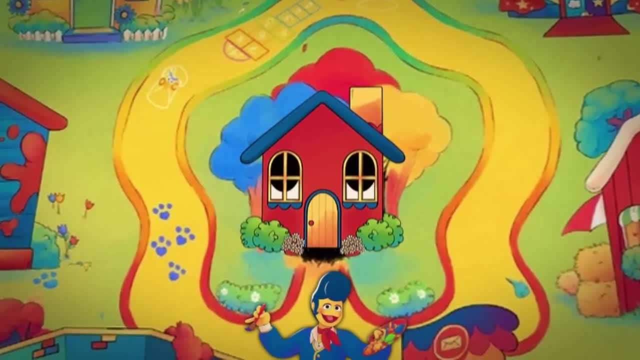 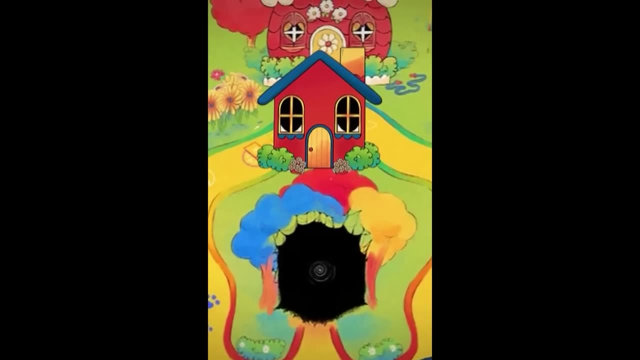 it's just Home And given that it's Wall-E's house and he's some kind of a cult leader, that strikes me as fairly suspicious, Especially when you check out the page on your phone, Because the image has to be resized for a mobile device. 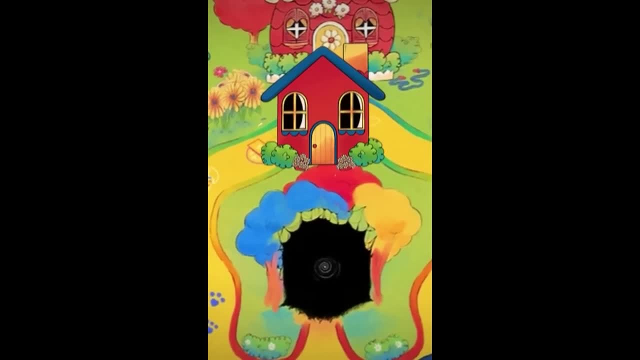 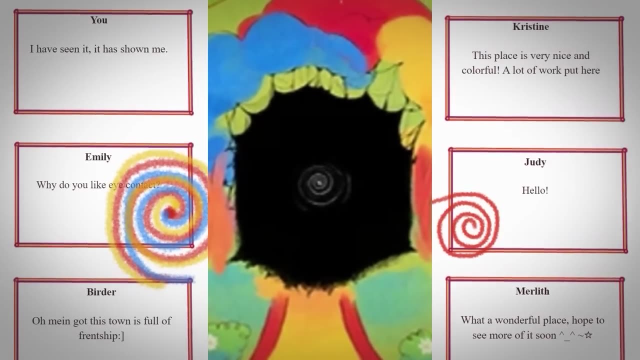 Home is no longer in the middle of the page. It's higher And, as a result, you see what's behind it: A black void with a single spiral in the middle, Just like the spirals that Wall-E is drawing into the guestbook. 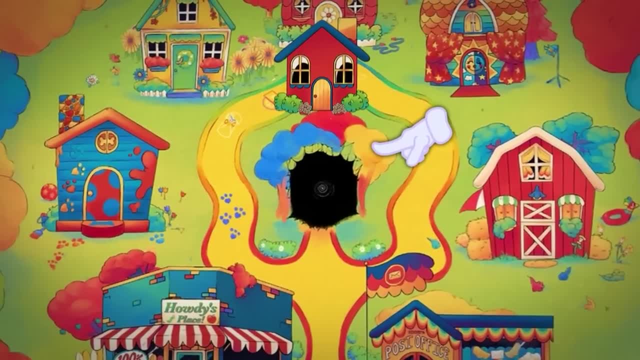 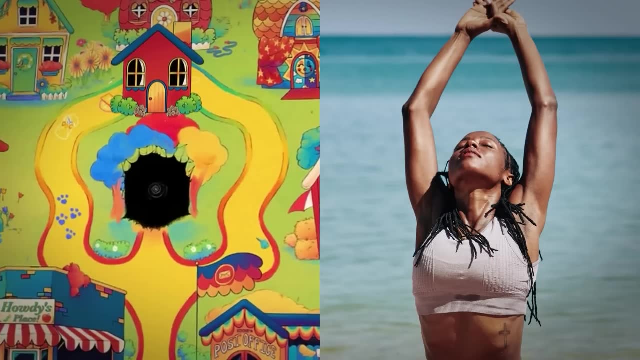 And while that is certainly disturbing, look at the whole image: The colorful trees in the middle, the paths leading to and from the void, and all around the neighborhood It almost looks like a person lifting their arms in an act of worship. Wall-E isn't the deity here. Home is. 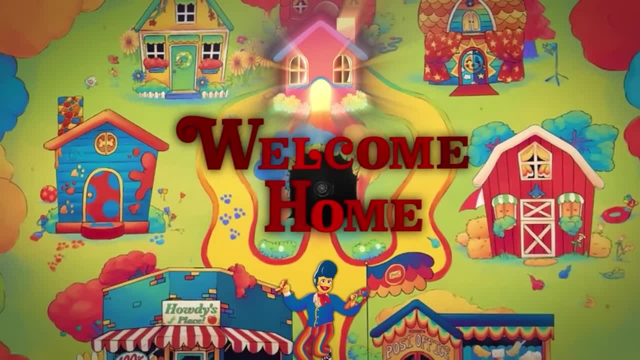 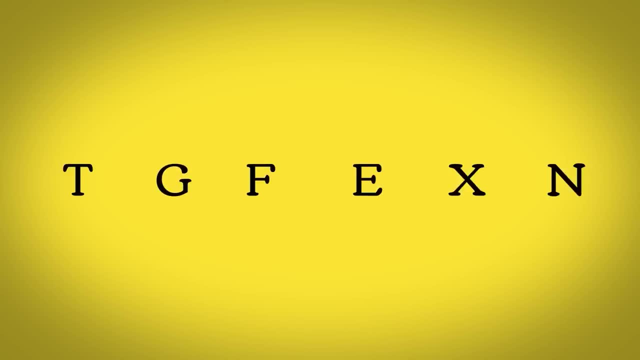 Wall-E is just the good and faithful servant. They are all welcoming Home. If you remember the letters that we used to find some of those hidden webpages at the top of the episode, there's a couple that I neglected to mention. If you put them in the order: Y-X-W-V-O-E. 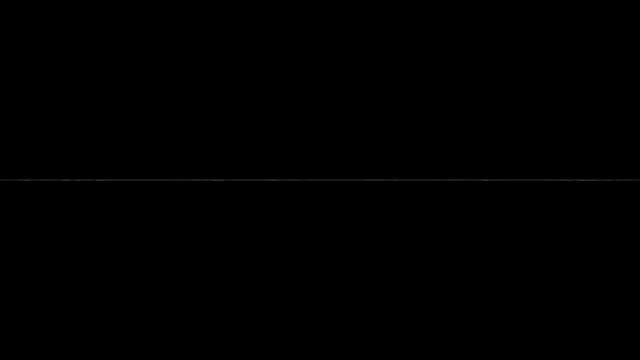 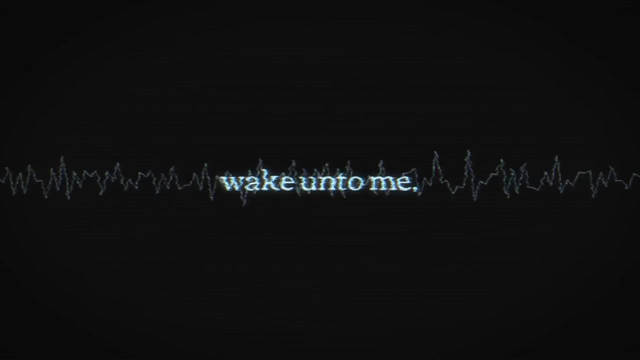 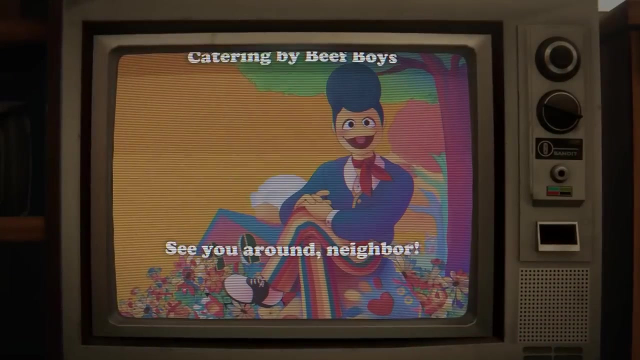 you'll find an error page, But click the telephone and suddenly we're treated to a rendition of the song Beautiful Dreamer In the world of Welcome Home nights symbolize the end of the episode. The neighbors would all go home, the children would turn off their TVs. 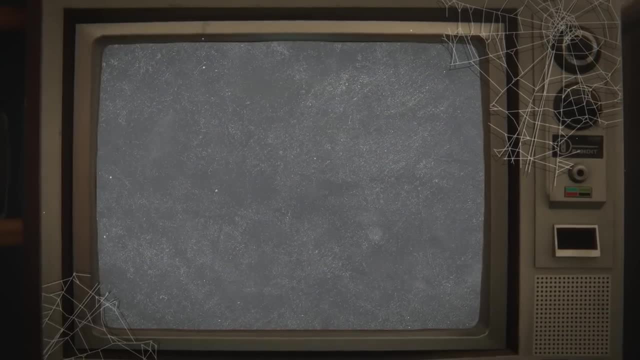 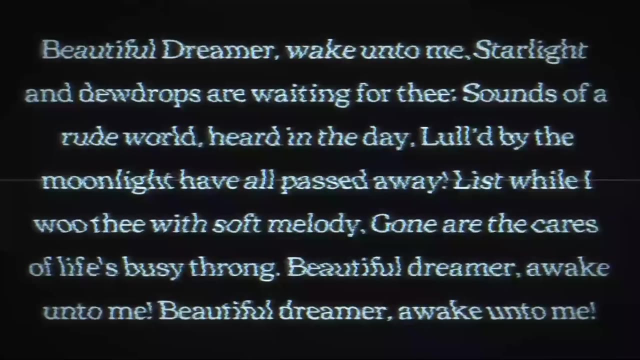 and the crew would retire for the night. The show, however, has been off the air for a very long time- Nearly 50 years- And so it's time for Home, the beautiful dreamer, to awaken once more, And we can be sure that this song is directed at Home. 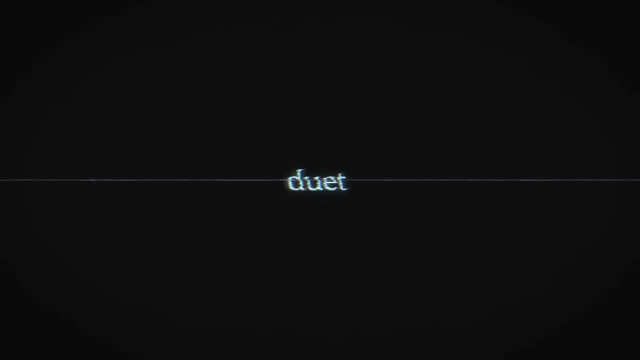 because, while the song is currently labeled as singing MP3 in the files, the webpage is labeled duets, But there's only one person singing, Or is there? If you listen a little further to the end of the song, you'll hear some banging sounds. 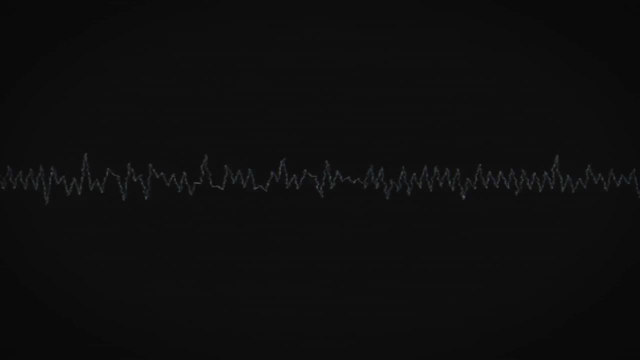 Do you like it? If we read Wall-E's bio, it says that Home talks using onomatopoeias. So these banging sounds are Home, responding to Wall-E's song, slowly awakening ready for revival. We don't exactly know what happened in 1974,. 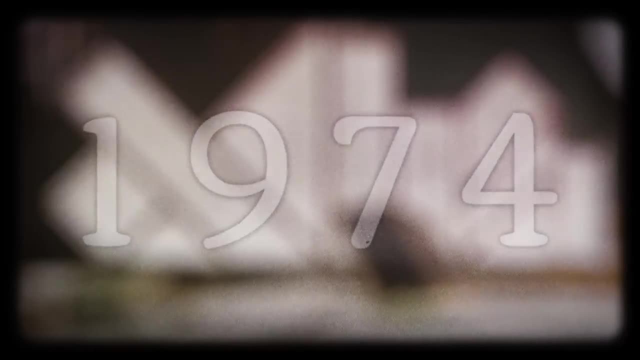 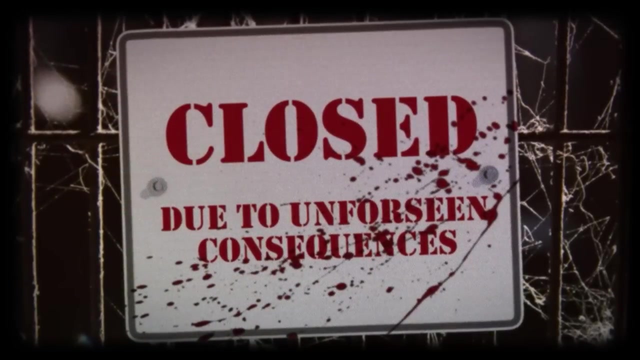 what caused the show to shut down and the production company to fall silent. but I've seen my fair share of indie horror to know that when you got sentient mascots and demonic entities, it's not gonna be a good one. Maybe the production company fell silent because many of their workers were killed? 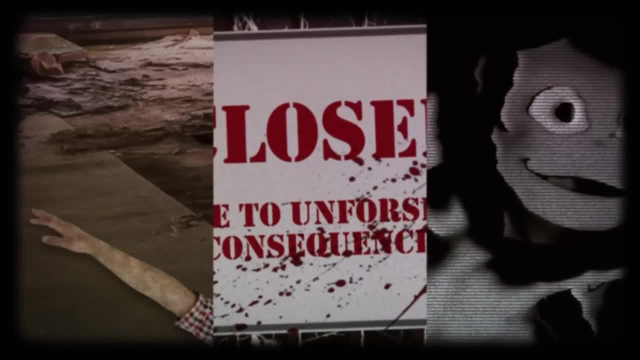 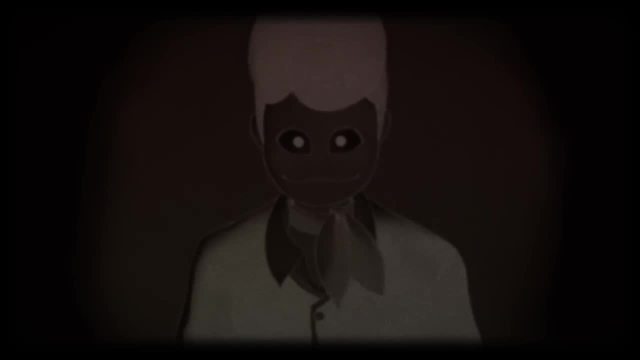 Maybe a ton of children died. Maybe Wall-E was able to possess them through the TV to serve whatever Home's motivation is. Whatever happened back then, it is gonna happen again. now that this exhibition is planned, Wall-E is regaining his influence, sharing these images to gather people together. 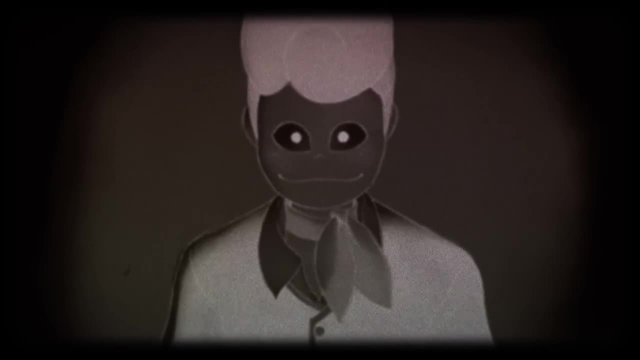 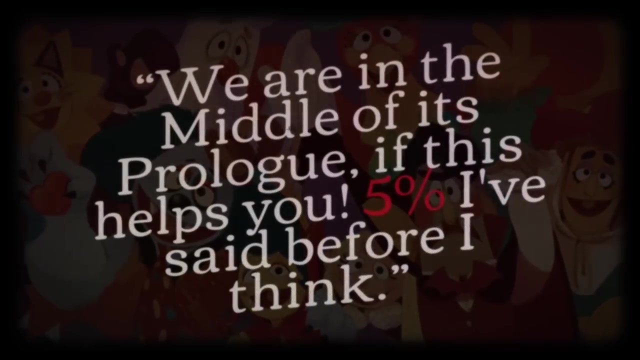 and slowly he will reawaken Home to continue, whatever their plan was half a century ago. The one thing I do know is that this story of Welcome Home has me hooked, Especially when you consider that Clown has said that we're only 5% into the project. 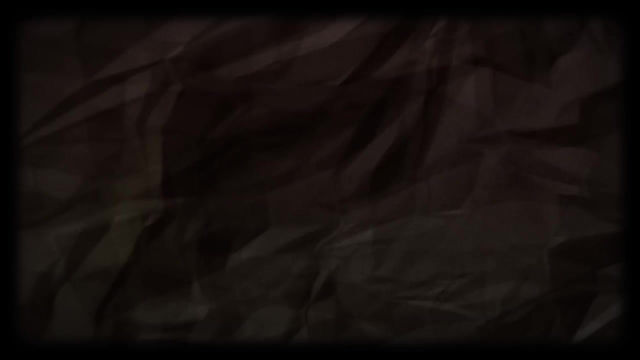 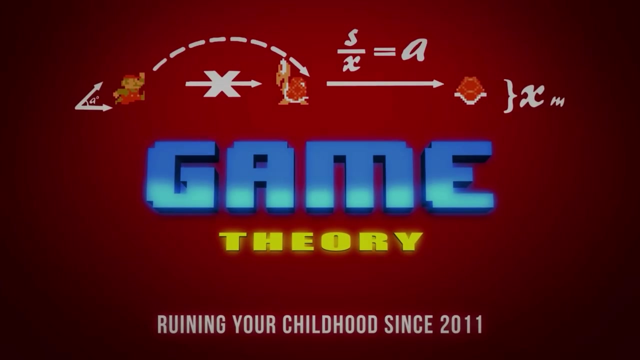 So until more is revealed, we wait. I suppose you could consider us the Neighborhood Watch. But hey, that's just a theory, A game theory. Thanks for watching. I hope you enjoyed this video. I'll see you in the next one. Bye. 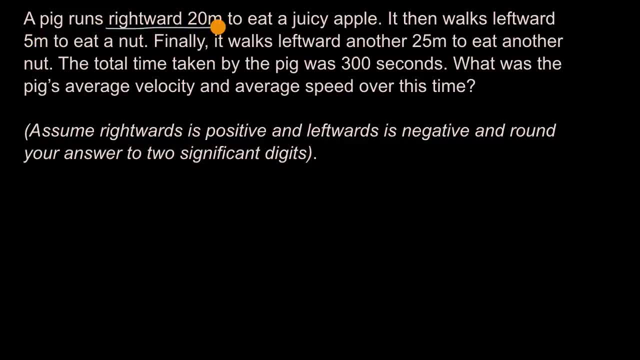 We are told. a pig runs rightward 20 meters to eat a juicy apple. It then walks leftward five meters to eat a nut. Finally, it walks leftward another 25 meters to eat another nut. The total time taken by the pig was 300 seconds. 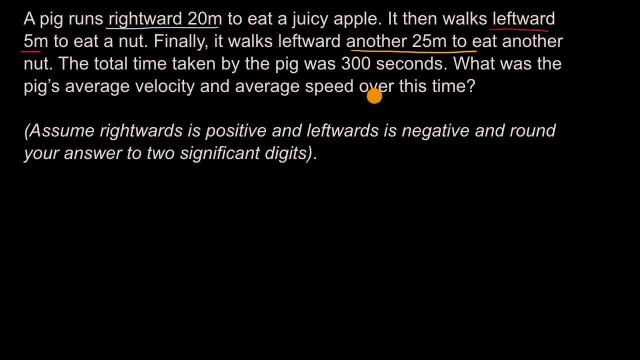 What was the pig's average velocity and average speed over this time? And assume rightwards is positive and leftwards is negative and round your answer to two significant digits. So pause this video and try to work it out on your own. All right, now let's do this together.